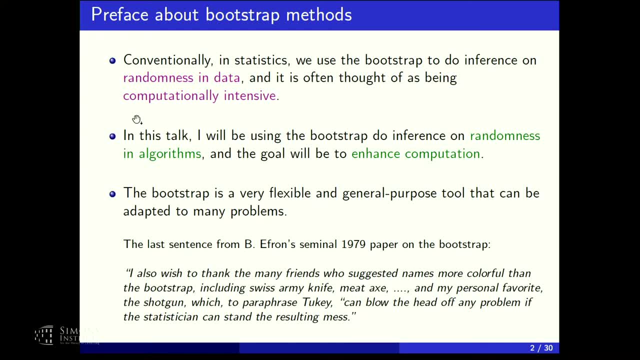 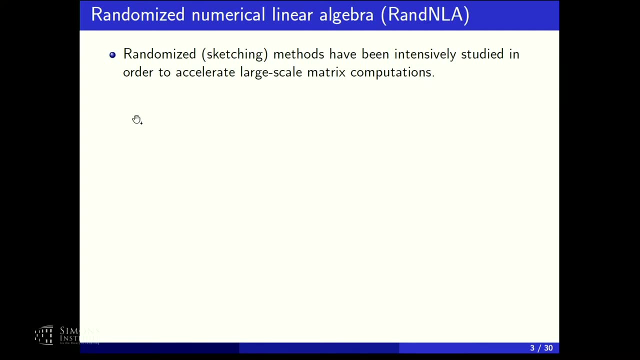 stand the resulting mess. So I think nowadays we can tolerate the mess a lot better than they could in 1979, just due to the fact that distributed computing is becoming ubiquitous. So I think the bootstrap's a pretty cool thing. I don't really need to go through this slide very carefully in light of everything that's been said in the. 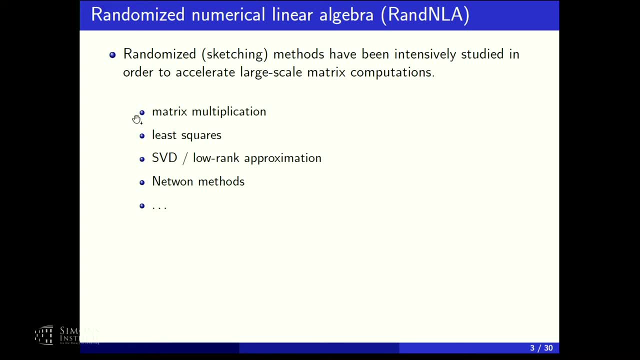 past two days. so we all know that randomized numerical linear algebra has been intensively studied now for quite a while and there have been highly optimized algorithms and so on. But of course, in exchange for getting these speedups over more traditional algorithms, we pay a price, which is we have to tolerate some. 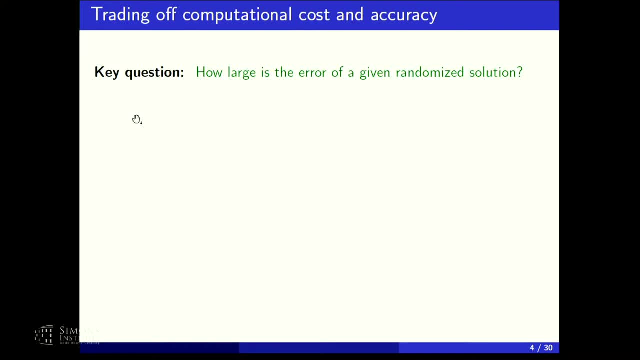 random error, All right, and this is the issue I really want to focus on. And so if we compute some randomized solution, how large is the error for that particular solution? OK, Not in the worst case, not in some other general sense for this particular solution. That's the error, that. 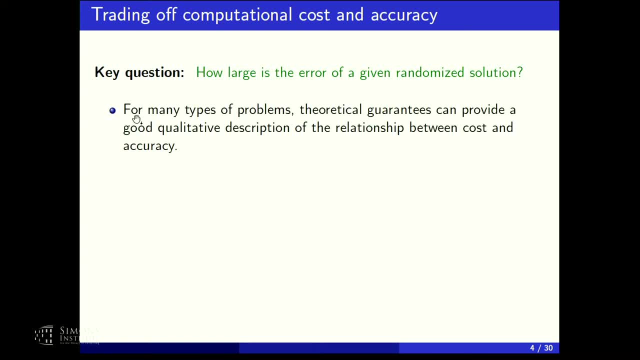 I want to study. So the prevailing sort of theoretical viewpoint in this area has been to derive theoretical bounds describing the errors of solutions, and this is a very useful thing. It gives us a lot of insight into the factors that the quality of the output, but there's some sort of essential limitations to 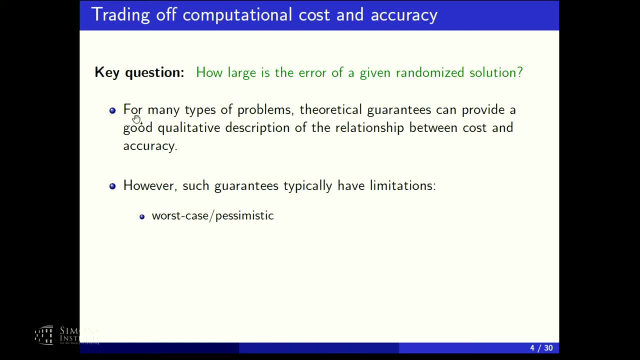 this kind of approach. so often, it's done from a worst-case point of view, so it may be pessimistic for any particular problem. The bounds often involve constants, which may be. even if you can whittle them down to something nice, they are often still conservative or, even worse, they could involve unknown. 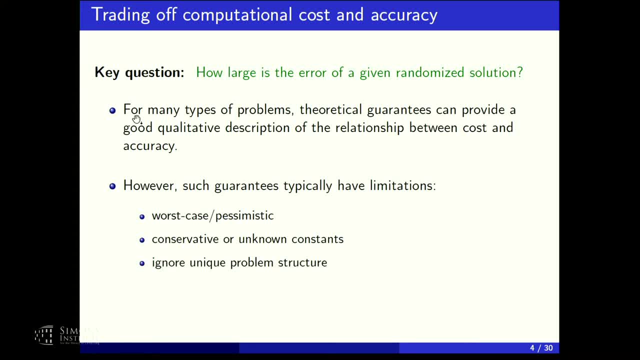 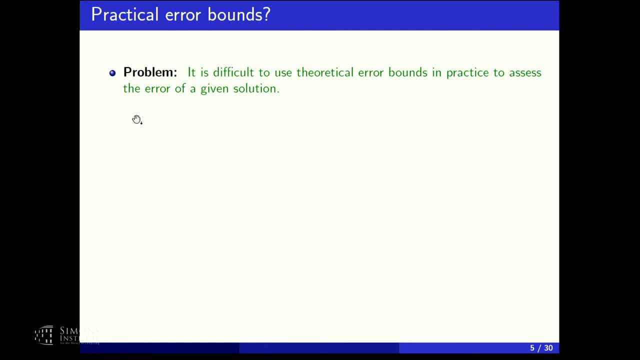 constants, and likewise they typically do not take advantage of the structure that may be unique to your given problem. so for these reasons, it's often difficult to use these theoretical bounds in any sort of numerical sense in a given problem, and so what I want to pursue is an alternative. so I want to numerically 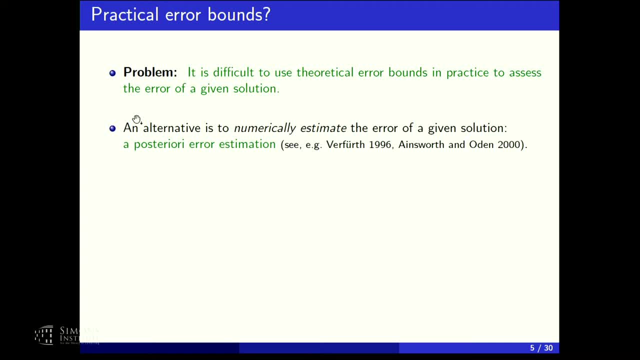 estimate the error of a given solution and in certain areas of applied math this approach has a name, it's it's often called a post Ori error estimation. so in areas like numerical PDEs are finite element methods. that in general you need a Michael D¡¡ message and then you need an 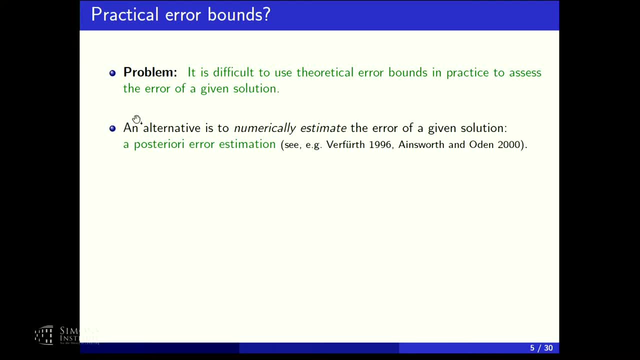 dataset that costs little but more Wat os, the��면 for the environment. that's often called a posterior error estimation. so it's in areas like methods. This is a fairly well-developed thing. There are even some textbooks written on it. In numerical linear algebra- randomized numerical linear algebra maybe not so much. There are. 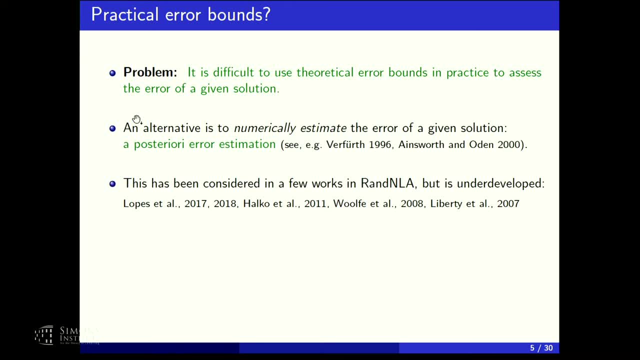 a handful of papers that have considered this at least a little bit And in fact, among these few references, some of the people are here, But nevertheless I would say that it's safe to say that this approach is underdeveloped and there's quite a bit of potential to explain. 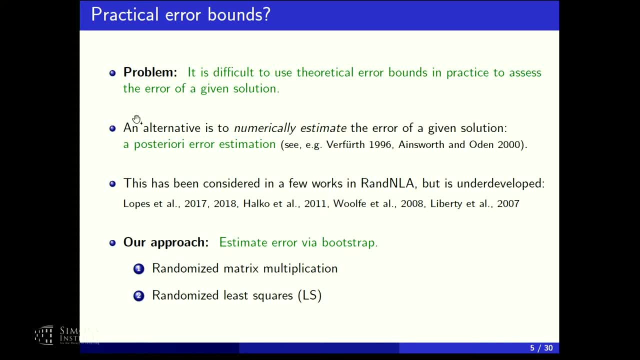 and explore what you can do with it in a broader variety of algorithms. So I'm just going to focus on two prototypical linear algebra methods or algorithms which are just matrix multiplication and least squares, And I'm going to break the talk into more. 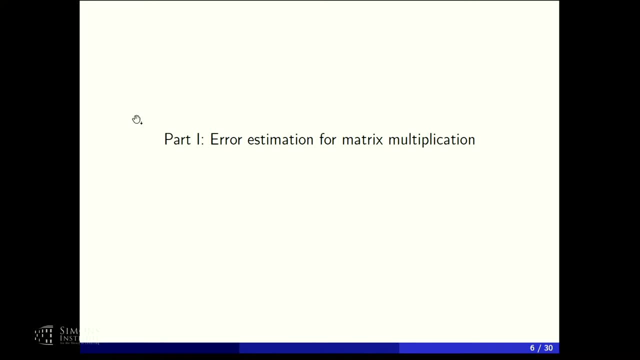 or less two disjoint pieces, OK, So I'll just outline the setup. So I have two extremely tall matrices, A and B. They're deterministic. OK, In all of the problems I'll consider the inputs I'm viewing as deterministic Even. 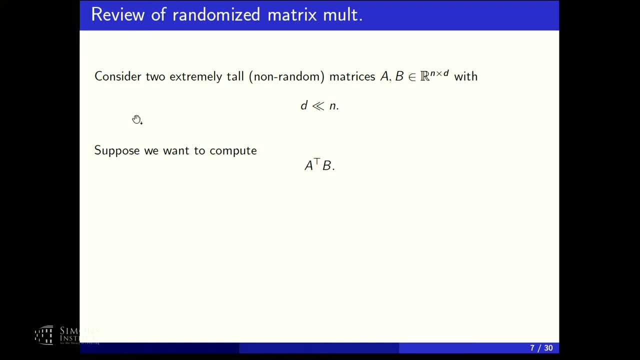 though they could obviously be data, I'm not going to consider that source of randomness. I'm only going to focus on the randomness in the algorithm and or the randomness in the bootstrap method that I'll propose. OK, So the number of rows is n. That's a very large number. The number of columns is d. 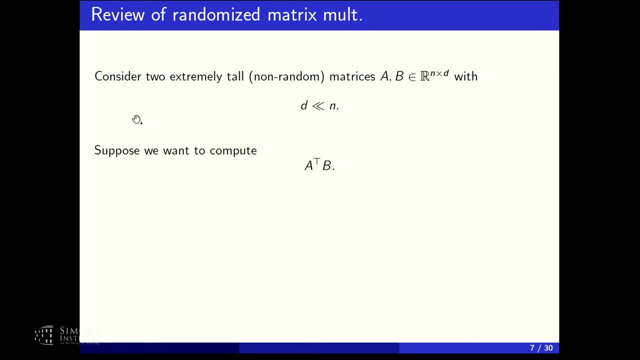 It's relatively small. compared to n, It could be large in the absolute sense. And let's say we want to compute A, transpose B. OK, All right, All right. So, as we know, the cost of ordinary matrix multiplication is n times d squared, And we want to bring that down, So we do, I guess. what's now? I guess. 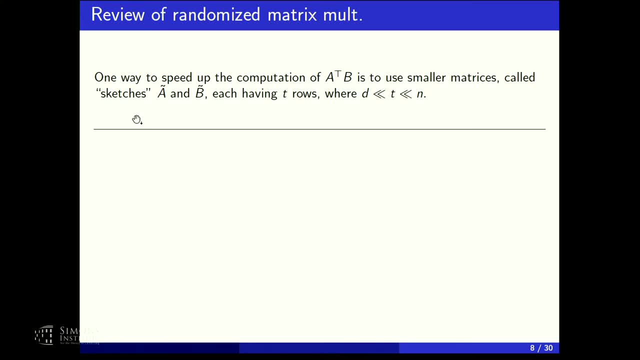 commonly known as sort of a sketch and solve kind of thing. So we'll form sketches out of the original matrices A and B. I'll use the letter t to denote the sketch size. So I'll bring the n rows down to t And I'll denote the sketches as A tilde and B tilde. 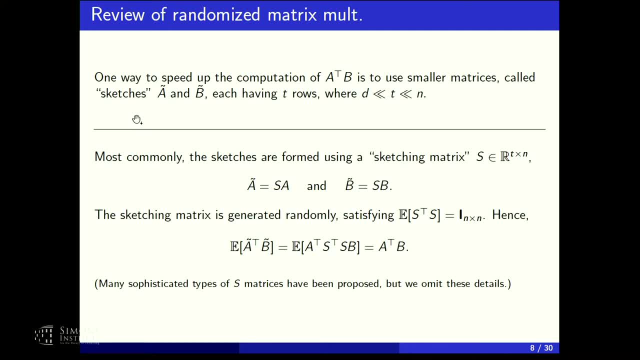 OK, And for the purposes of the bootstrap, there's really only two basic properties that I'll need for the sketching matrix. So I'll just need that the expected gram matrix is the identity and that the rows of the sketching matrix are essentially independent. OK, Conceptually. 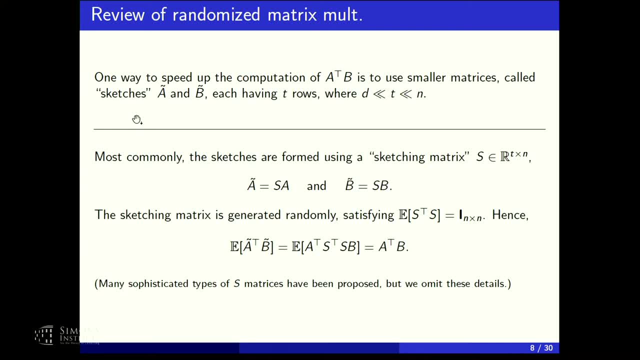 that's really all that matters. When you look into the fine-grained details, when you derive bounds and so on, there are some different technical consequences for different choices of sketching matrices. But I think that's sort of a second-order consideration. 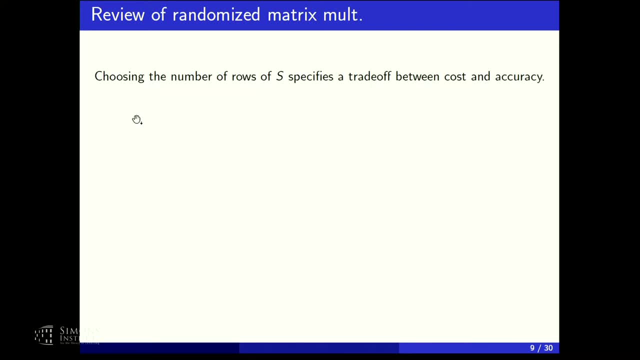 OK, All right. So how do we choose t? OK, So there's a direct relationship between the choice of t and the quality of the sketch product. All right, So of course, the quality is going to improve as t gets bigger, And that's essentially a consequence of the law. 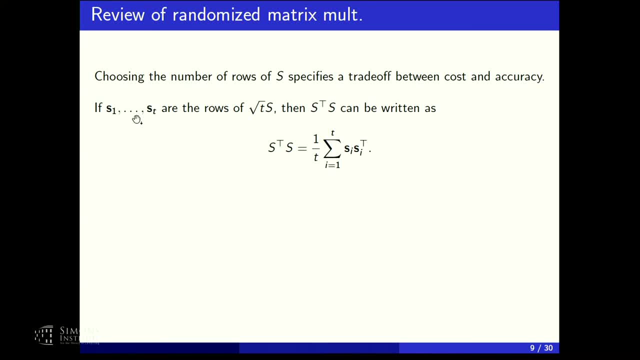 of large numbers. So if we expand the gram matrix out as a sample average of rank 1 matrices, independent rank 1 matrices, OK, And we know that the expectations identity, this is going to get closer and closer to the identity with high probability And therefore the sketch product is going to get closer. 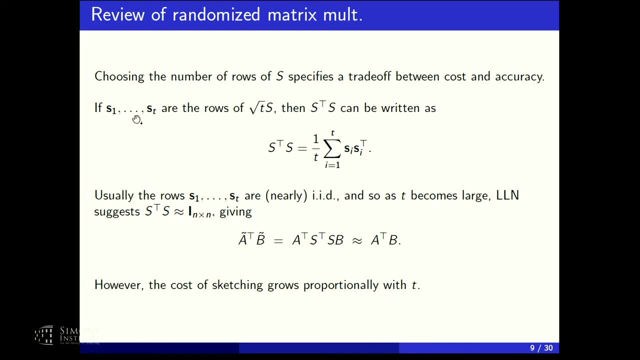 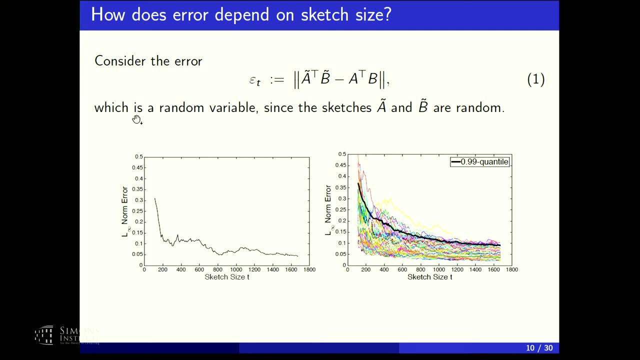 and closer to the true one. All right, So that's clear at a conceptual level, But what does this actually look like in a real example? I think this plot gives a lot of insight into what's going on at a sort of- in a sort of- statistical way. So let's focus on the left. 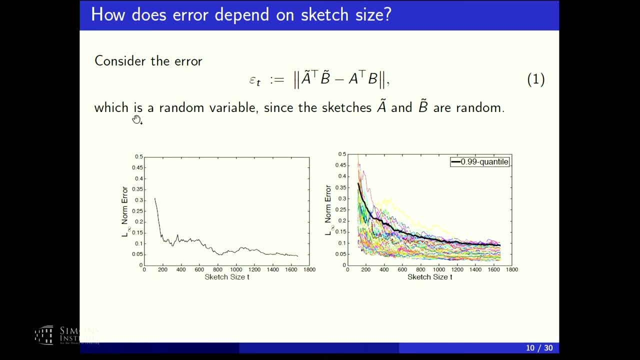 plot first. OK, The way I've generated this plot is as follows. I incrementally add one row at a time to a sketching matrix. Each time I add a row, I compute the exact error for that particular sketch against the true product. 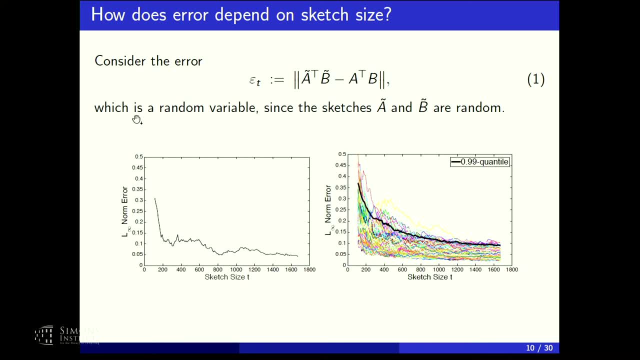 Of course, this is not something you can do in practice. This is just to illustrate what's going on. As you expect, the error generally improves as the sketch size gets bigger, but there's some fluctuations along the way. Now you can imagine repeating that entire experiment many, many times, and that's what 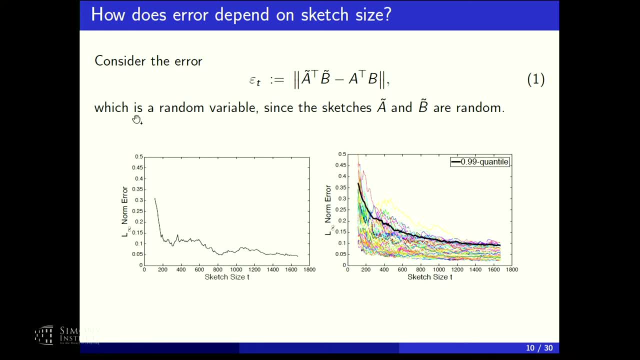 the right plot shows. The right plot shows many independent copies of the sample path that's on the left. You see, there's actually quite a bit of variation. Another way to think of this is each person in this room could have their own sample path. 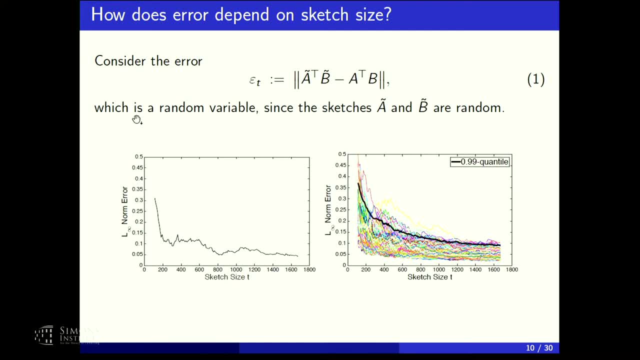 This reflects the quality of all of our sketch estimators in aggregate At any given sketch size. what any one of us wants to know is: Okay, What's an appropriate error level, such that I'm likely to be below that for some tunable probability? 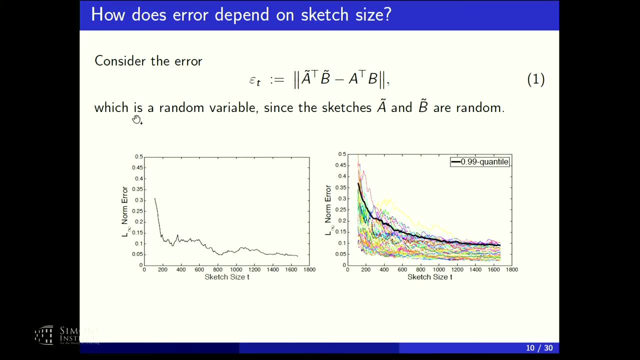 There's a name for that. It's called a quantile, or let's say, the 99th percentile. That's what the thick black curve is. I think this quantile function or quantile curve is a very useful way of thinking about. 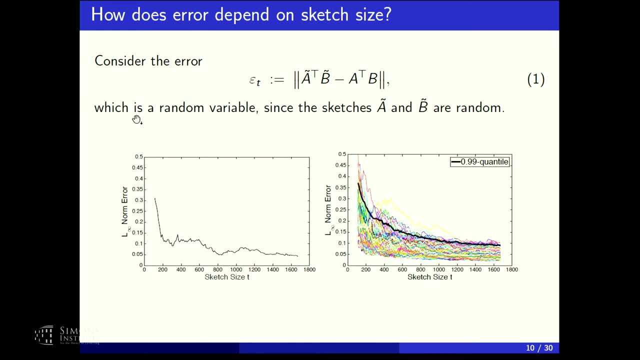 the trade-off in a very quantifiable and estimable way. I'm going to use the letter epsilon sub t to denote the random error variable. Yeah, Does it look very different if you plot just for being this one error? I think conceptually the choice of the norm doesn't matter so much. 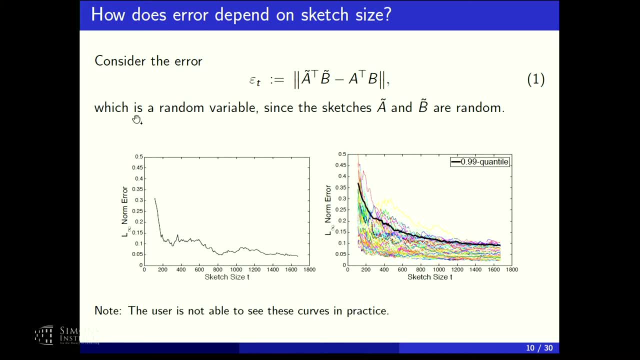 The scaling will change et cetera. but I would say, as long as the norm or error functional more generally, is a smooth functional, then this kind of picture arises. In fact this is a very, very generic sort of thing I've done. 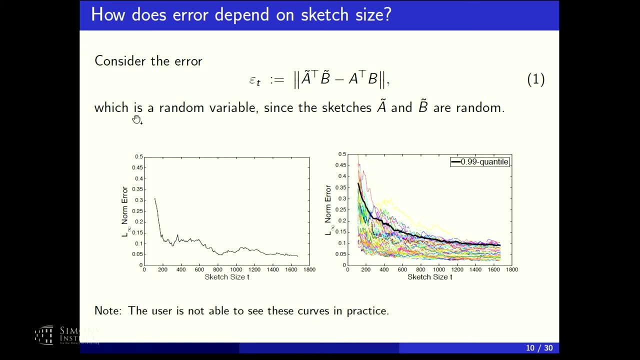 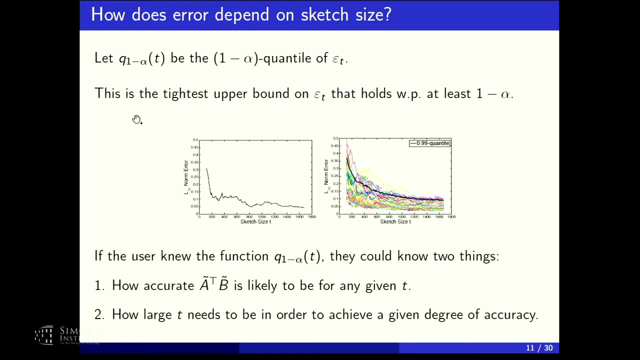 Okay, Okay, I've done things with random forests, I've done things with least squares. This is sort of very generic, Okay, All right, I'm going to call the quantile function q sub one minus alpha of t, so the probability. 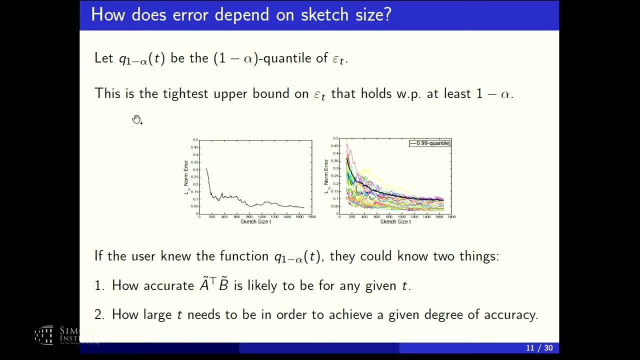 that I'd like to have for an error bound, let's say, is one minus alpha. If we had access to this quantile function, we could do two things with it. For a given sketch size, it gives us a particular bound with high probability. 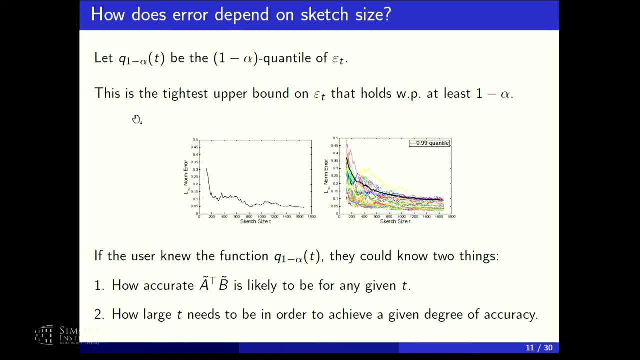 But there's another way we could use it, which is sort of in a predictive sense. So if we have some error tolerance that we'd like to achieve, this quantile function will allow us to look ahead and forecast what sketch size we'll need to get to in order to achieve. 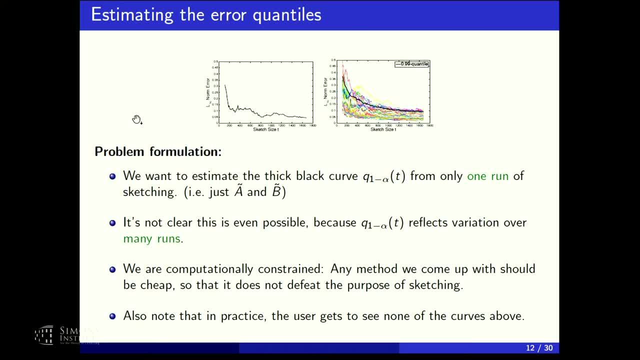 that. So both of these, I think, are interesting And this is what I'd like to estimate. So that's sort of the well-defined statistical problem that I'm proposing to solve. I want to estimate this function, And here's why it's not easy. 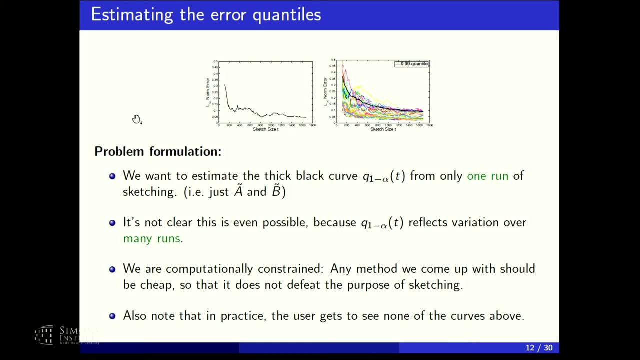 Okay, So I constructed this thick black curve based, hypothetically, upon many experiments, right? But in real life we only get one A tilde and one B tilde generally, or at least that's what we want. We only want to run the sketching algorithm once. 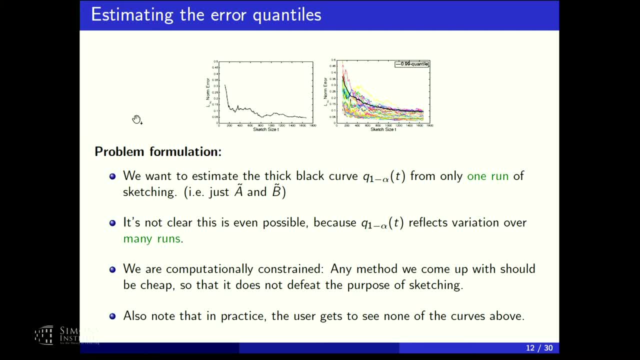 So it might seem almost impossible that you could approximate this thing. that comes from many repeated experiments, just from a single experiment, And that possibility is, in a sense, what is so remarkable about the bootstrap. Okay, So the bootstrap is what makes it possible to do that. 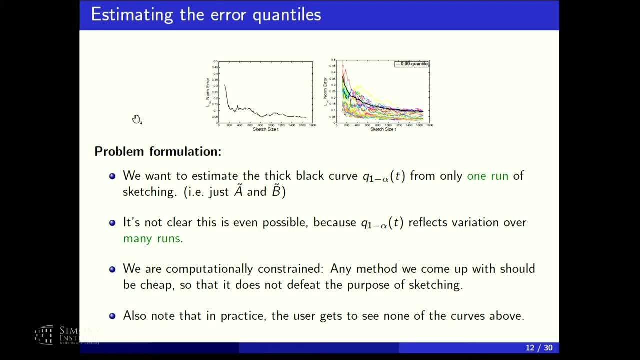 And another important consideration is that we're computationally constrained. right, I don't have an infinite amount of resources to compute this quantile function. even if I come up with something clever, It needs to be cheap enough so that it doesn't outweigh the benefit of doing sketching in. 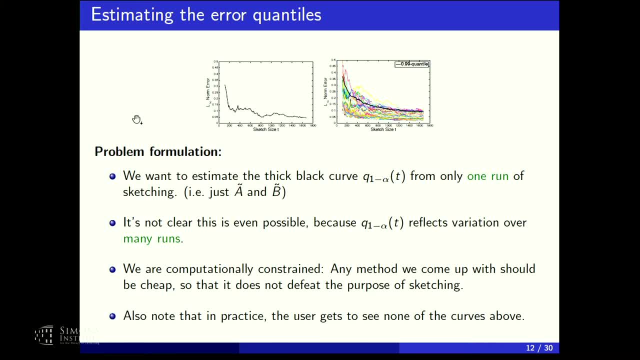 the first place. Okay, So I'll definitely keep track of this cost as things go along. And again, just to make this point clear, we never get to see any of these curves in practice. okay, So this is just for illustration. 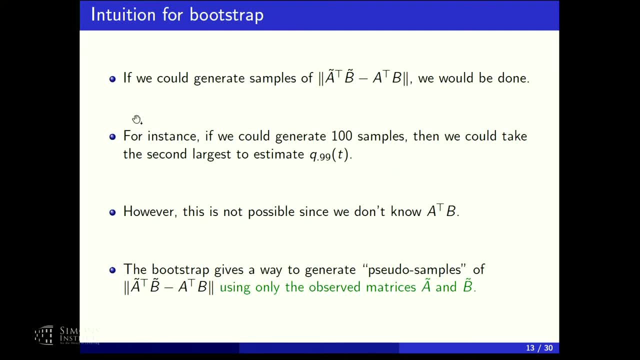 All right. So let me give you just a little bit of intuition for how the bootstrap algorithm will work. So let's imagine for the moment we could generate independent copies of the error variable. Of course we can't do that, in particular because it depends on the true product. 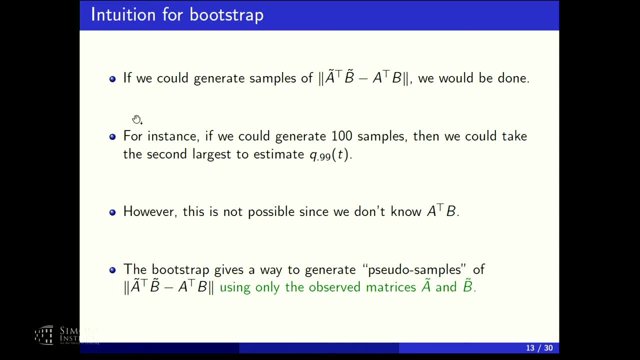 But if we could- let's say we could- generate 100 samples, well, we could take the second largest of them And that would be a natural estimate of the 90. That would be quite effective. Of course, we can't do that. 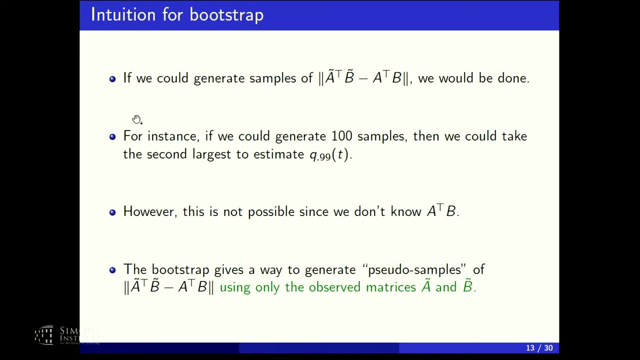 So, in essence, what the bootstrap tries to do is to generate pseudo-samples of this variable, plain and simple, And then, once we generate enough pseudo-samples, we'll take the quantile of those. All right, So here's the algorithm. 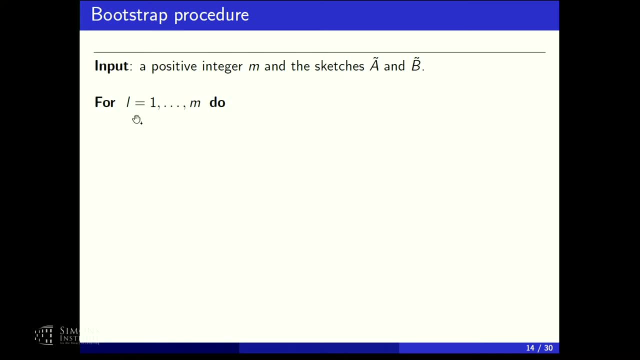 I could fit it easily all in one slide. So the input is an integer m, That's the number of samples I'm going to generate, And then the only other inputs are just the a tilde and the b tilde. All right, 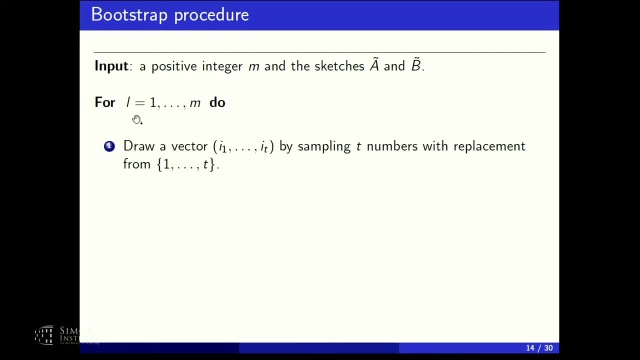 So here's the loop: I'll draw a vector of numbers, without replacement, from the set 1 through t. I'll take those indices and then I'll plug them into my sketches And I'll use those to form, or I'll take rather the rows of a tilde and b tilde, indexed by 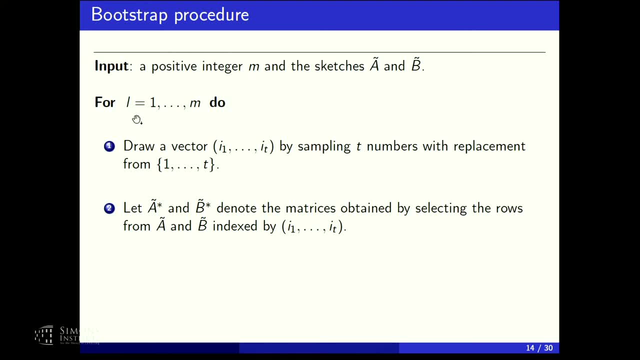 these random integers And that will give me two new matrices: a tilde star and b tilde star. So there's going to be replicates of some of the rows of a tilde and the b tilde in the starred versions Then. 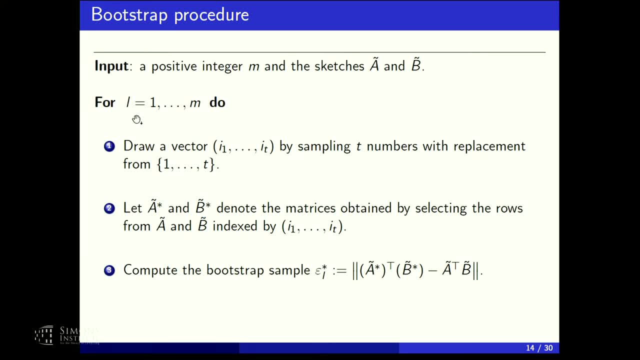 I'll take the norm of the difference between the starred product and the unstarred one And I'll view this as a pseudo-sample. So for each iteration of the loop I get one of these starred pseudo-samples. Then, after the loop is done, I take the desired quantile of those samples. 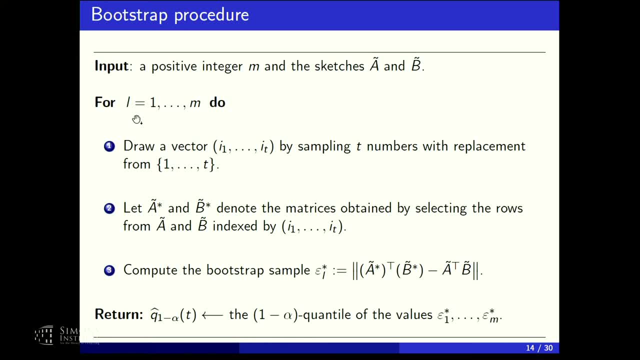 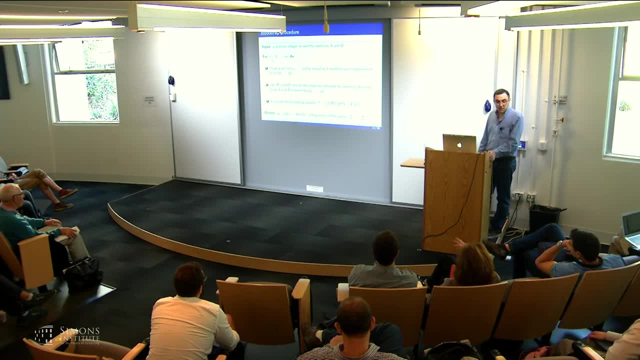 So this is the whole thing. It's really that simple, So maybe I should pause for just a moment in case there are any questions. Yeah, I have a stupid question: Why do you take the quantile? Why don't you just look at everything? 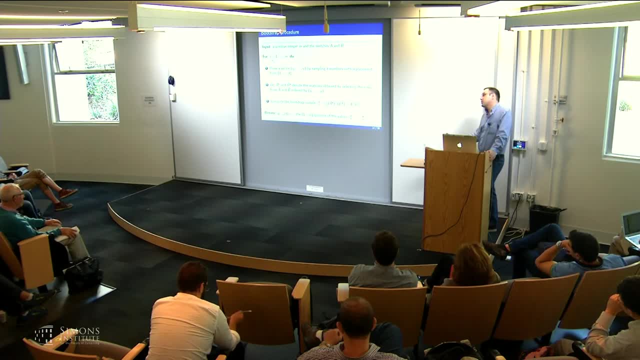 So I mean, I guess it depends on how you want to formulate the problem. So there are other ways. certainly You could look at variance instead of quantiles. That makes a lot of sense too. But I mean, if we agree that our goal is to estimate that population-level quantile function, 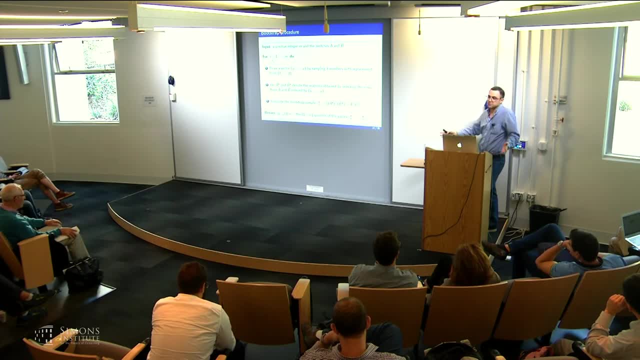 then taking the empirical quantile is sort of a natural thing to do, But there are certainly other things you could try. So, Yeah, So is it possible that you just regenerate many replicates? Yeah, So if you do the simplification of the sketching matrix, then you get A star rather than you. 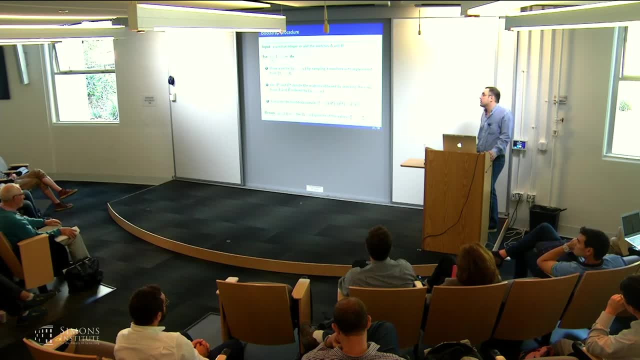 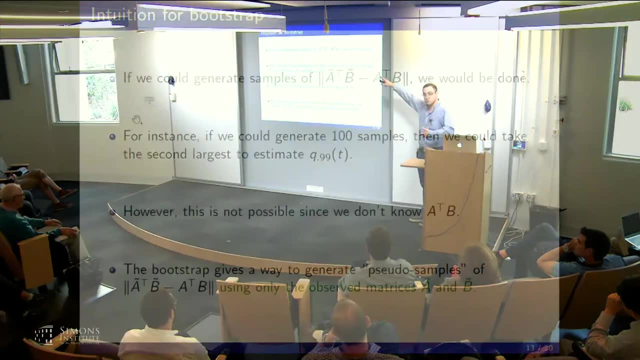 do a subsampling Right, But So, indeed, So that would almost. that would basically be what I was mentioning here. So if you, so you're saying, do actual sketching many times, Yeah, But the center is not A, transpose B, it's A2.. 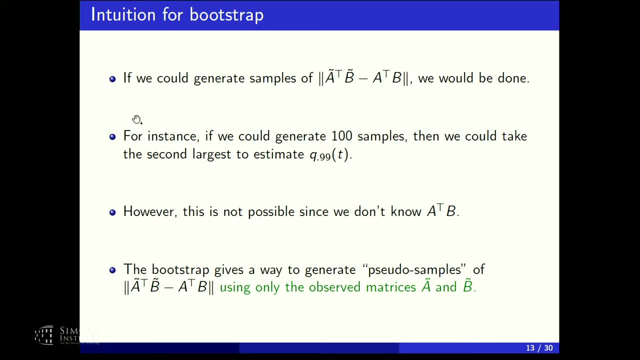 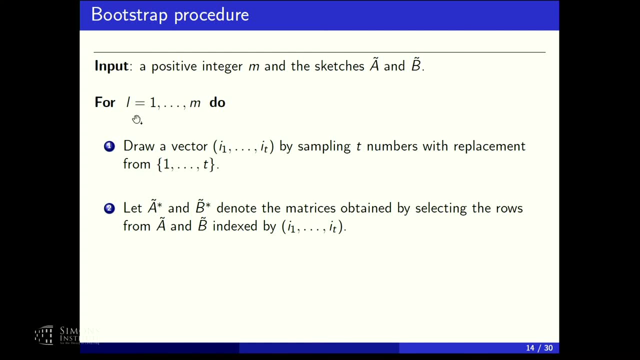 Oh, I see what you mean. Yes, Yes, you could do that. I believe, though, that the resampling is actually much cheaper, And we'll get into that. We'll get into that, maybe more in a second. Yes. 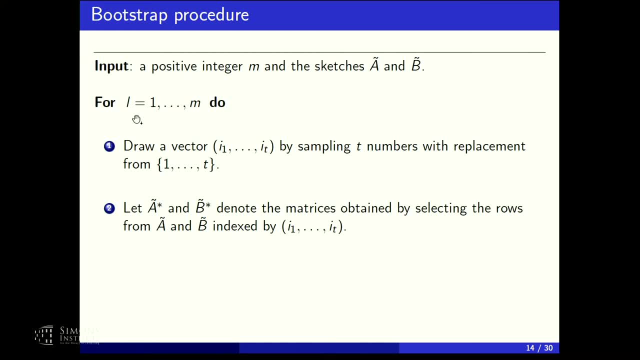 So in particular, yeah, you're not going to have to generate a new sketching matrix, You're not going to have to do any new matrix multiplication with a new sketching matrix. That's kind of baked into the sampling mechanism. Yes, 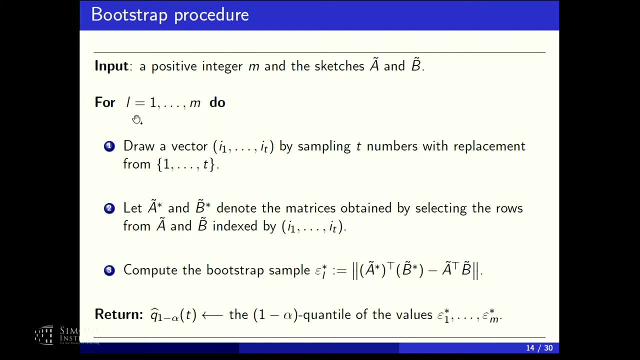 Also, your problem definition was to find out the accuracy of k-theta, B-theta, right. So his thing wouldn't really find the accuracy of this particular sketch, It would just find out the efficacy of sketching k-theta. It would effectively give me independent copies of that variable roughly. 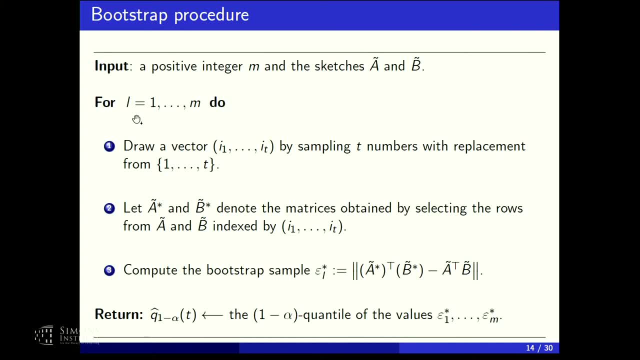 So I could imagine that working, but it wouldn't. indeed, it wouldn't give me an error estimate for this particular sketch, but it would give some reasonable way of approximating the quantile function. OK, So we'll just move on. 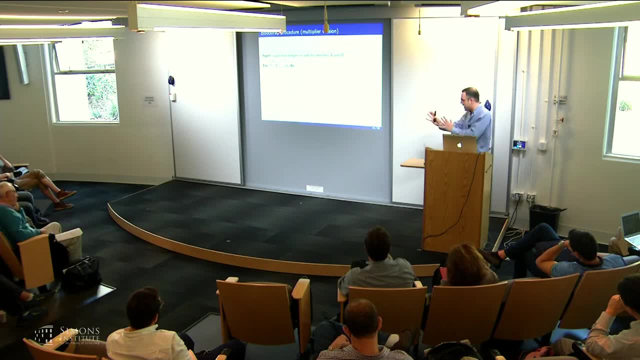 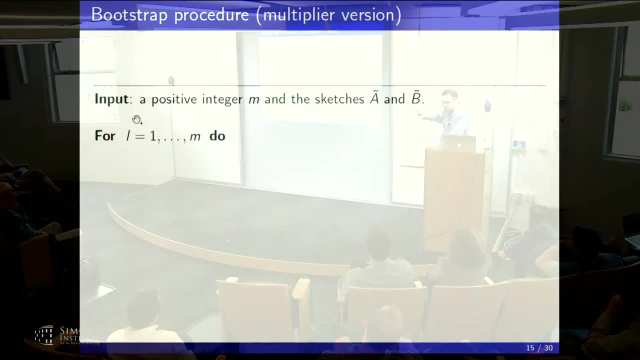 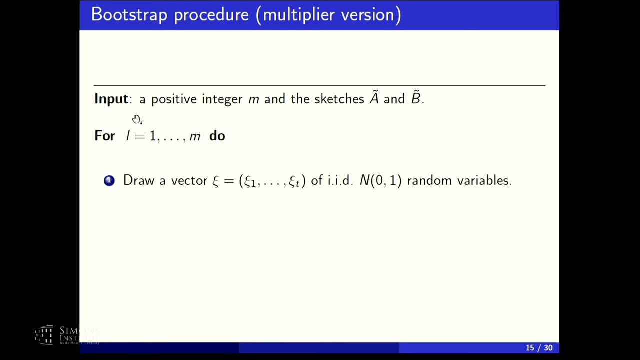 All right. So just to be accurate in how I present this project In the paper we analyze a slightly different version, So there's many flavors of bootstrap, if you will. So this is what's sometimes called the multiplier bootstrap in the statistics literature. 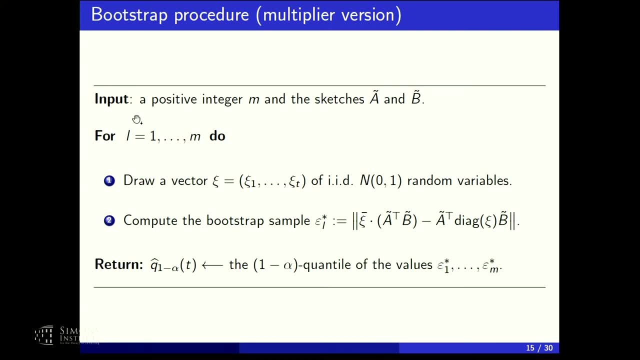 At a conceptual level, there's not really that much stuff that's different going on. In essence, the sampling is done using Gaussian variables. This is really just for convenience of analysis. If you do experiments, the results are effectively the same, So I'm just mentioning that. 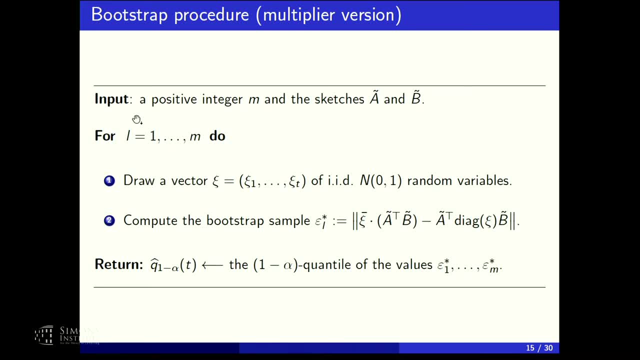 So, just so you don't get confused, If you look up the paper And there are some interesting differences, but at a high level this is not so different. So I won't go into the details, but there's a relatively simple way to see why this is. 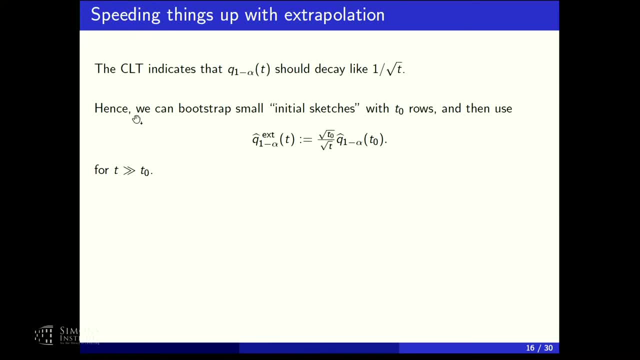 mimicking the previous bootstrap sample. OK, So now I have an algorithm, but how much does it cost? So what I want to argue here is that there's a really simple but effective way to dramatically reduce the cost of this. This is called the. 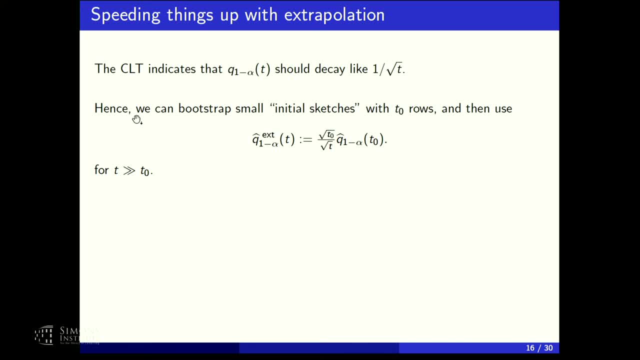 So the thing I'm getting at here is closely related to Richardson extrapolation. So the central limit theorem tells us that this quantile function should scale like 1 over square root of t, And that's really useful, Because what it means is if we could estimate a point very 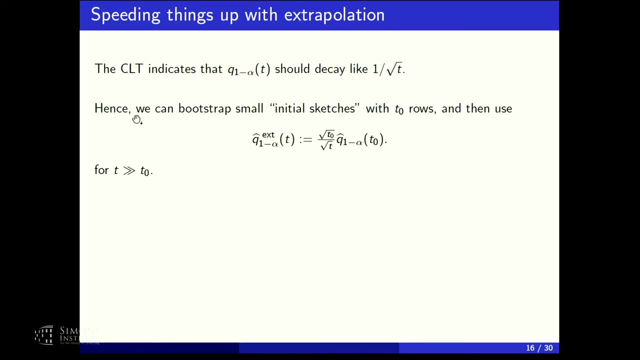 early on on this quantile curve. then we can just rescale to get everything thereafter. And what's kind of amazing is that as simple as that is. it works really well. So let's say, I generate some little sketches of size t-naught. 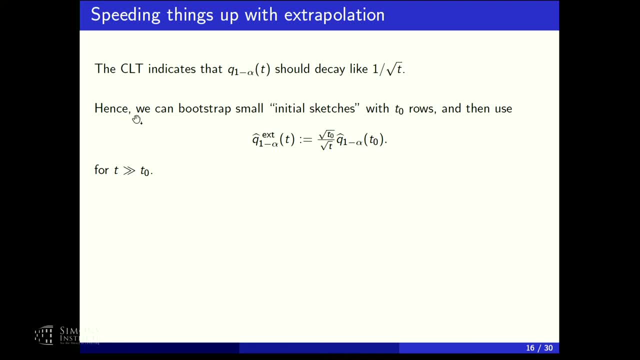 Those are going to be poor sketches, but I can still apply the bootstrap to those and get an estimate And then I just rescale for all t that are larger. So basically I would be estimating a point here, even though ultimately I'd probably. 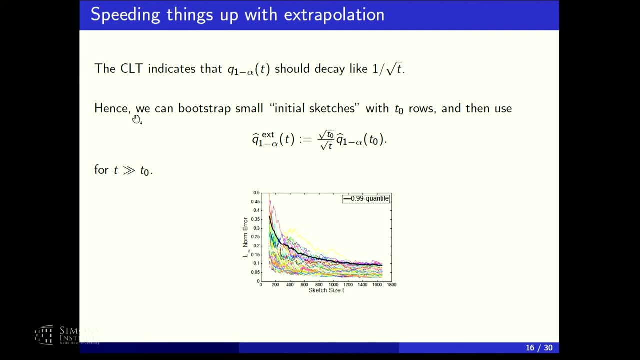 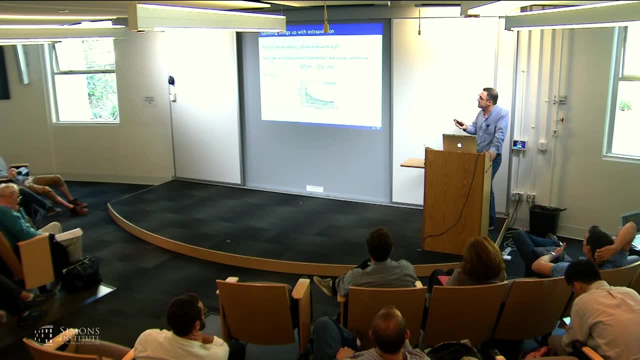 want a sketch size out there, So this t-naught is just sort of an expedient. Yes, It's only holding, because your n is assumed to go to infinity, right, Right? So this is a delicate question. I mean the t-naught needs to be of some moderate size, right? 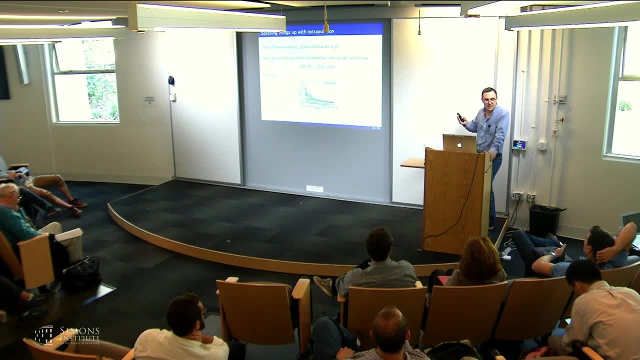 You want t-naught to be maybe at least 50 or 100.. It doesn't need to be huge, but it can't be just one. I'm saying you apply instantiations of the central limit theorem, chernoff-Hefti type. 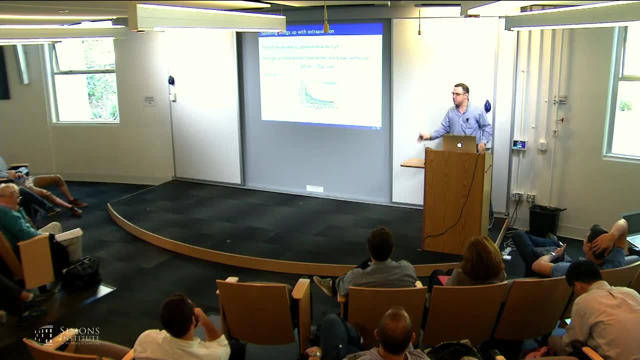 bounds here, Right. So I'll have a few comments about the analysis later. So the analysis involves a lot of things, but we can get into that All right. So let's be a little bit more detailed about the cost. So the cost of sort of generic sketching algorithms for matrix multiplication looks something. 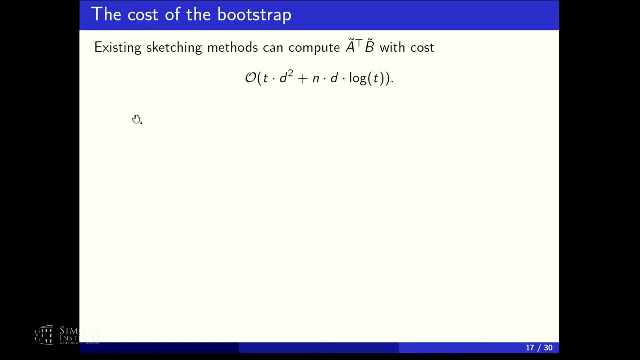 like this. So you have the cost of doing ordinary matrix multiplication on the sketches, And then you have this additional term that comes from implementing the sketches. So, for instance, in the case of randomized Hadamard, that's what the second term looks. 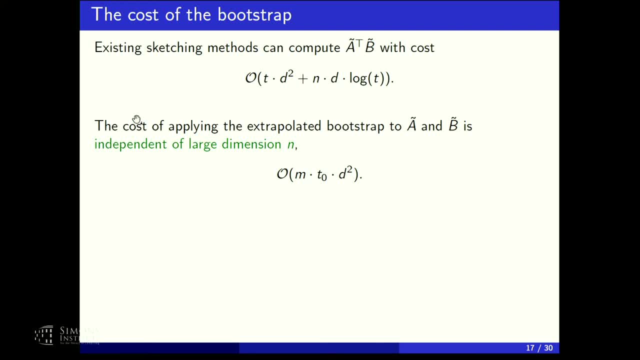 like, And this is the cost of the bootstrap. So at each iteration of the bootstrap loop I do ordinary matrix multiplication And that gives me the t-naught times d squared, And then I do that m times. So basically what I want is for this cost to be no greater than the first one. 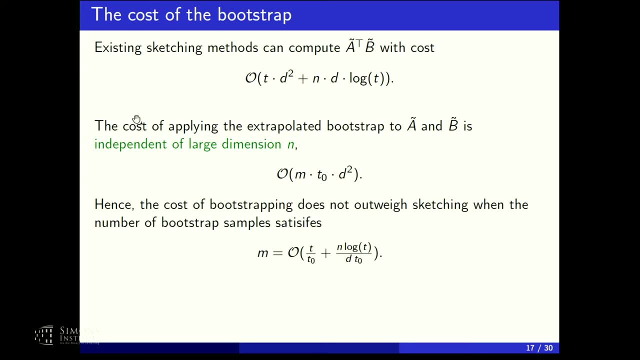 And that happens as long as the number of bootstrap samples is not too large. OK, So here you can see why the extrapolation helps. because it says that as long as the initial sketch size is relatively small compared to what I'll ultimately need for an accurate 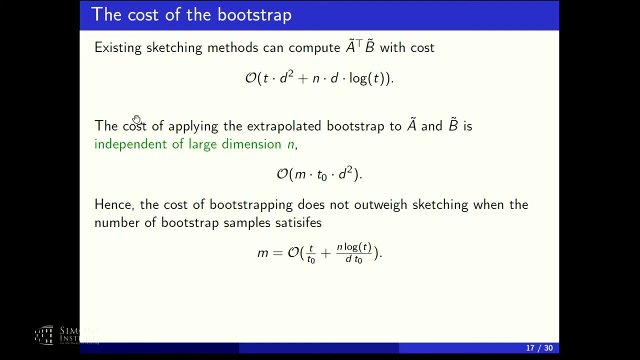 sketch, then that gives me quite a bit of runway for picking a decent number of bootstrap samples. And what's empirically nice- I'm just making an empirical statement here- is that in a lot of problems 20 bootstrap samples is perfectly adequate. 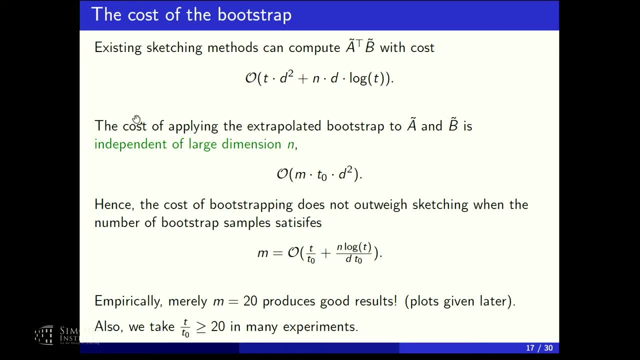 OK, So this You know. There's no, There's nothing sneaky going on here. OK, So it's. In fact, you could almost think of the number of bootstrap samples as being 0 of 1 for practical purposes. 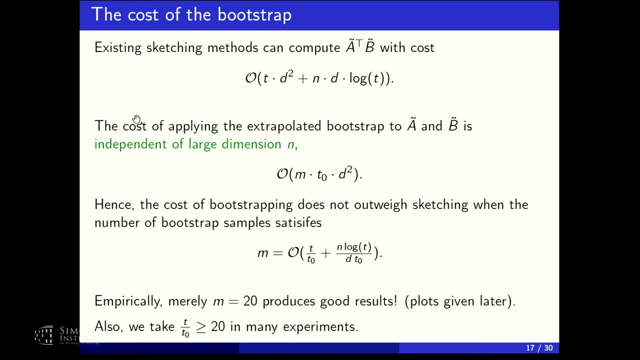 Maybe log or something OK. And furthermore, we're assuming n is large, right? So if n is much, much larger than d times a small initial sketch size, we're in good shape. So Yeah, How are you supposed to estimate the 99th percentile with only 20 samples? 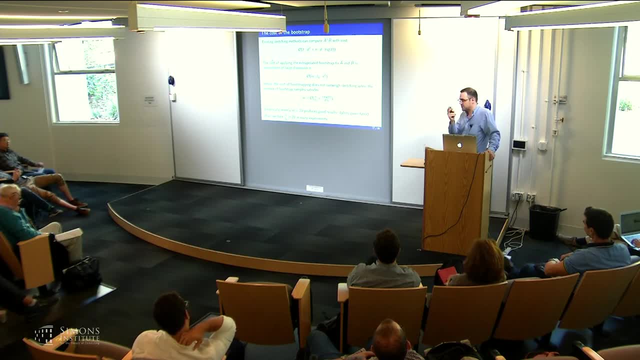 Oh, So Yeah, So this Yeah, So you can use an interpolation rule. So I think the second largest among 20 samples is going to be the 97th or 8th. It's going to be- It's not going to be quite- 99.. 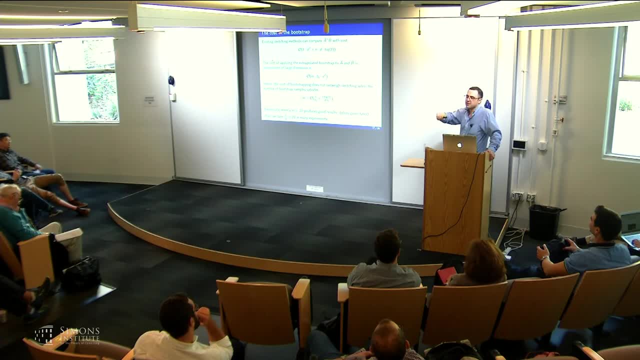 But there's a. There's a, There's a. If you use MATLAB or something, there are simple interpolation rules to get the 99.. It's a. This is a very minor detail, But indeed that's a legitimate point. 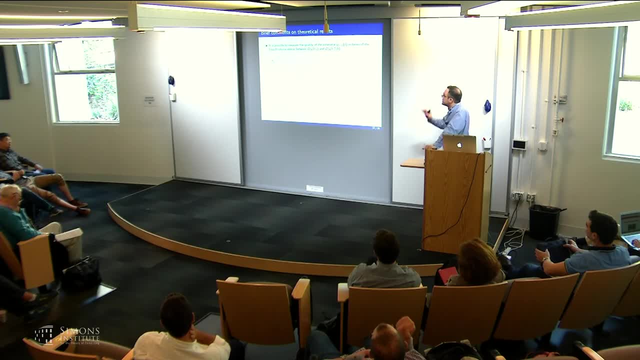 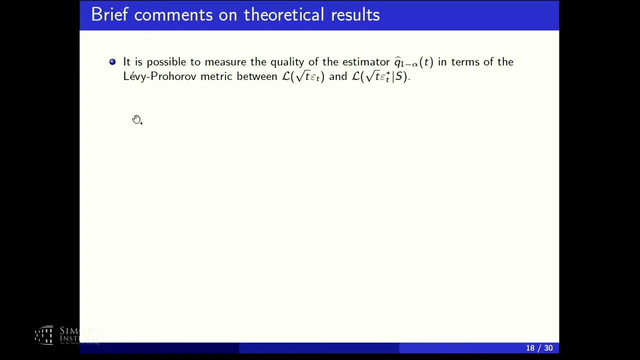 So, OK, I'll just say a few comments about the theory. There's a lot that could be said about the results in this paper And in fact most of the paper is theoretical. So to formulate the perform or to describe the performance of the bootstrap in a non-asymptotic 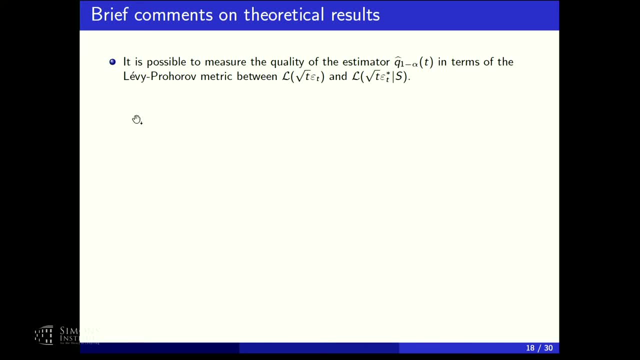 way sort of requires some care. So here's kind of a natural way of doing that. So I have a random variable whose distribution I'm interested in And I can consider the distribution of the bootstrap sample conditionally on the sketch that I drew. 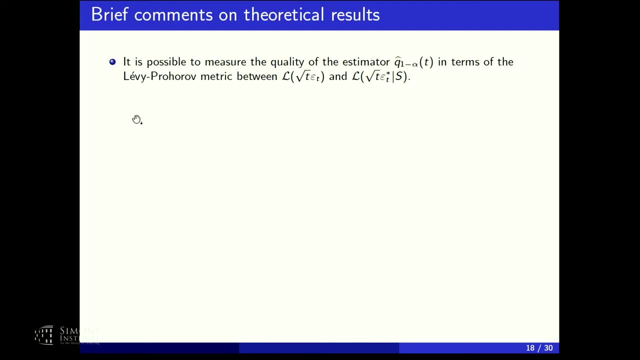 And if you compare those two distributions in a metric, there's typically a direct way of relating that to the distance between their quantiles, And I scaled them by a factor of square root of t, just in the interest of making comparisons with central limit theorem. 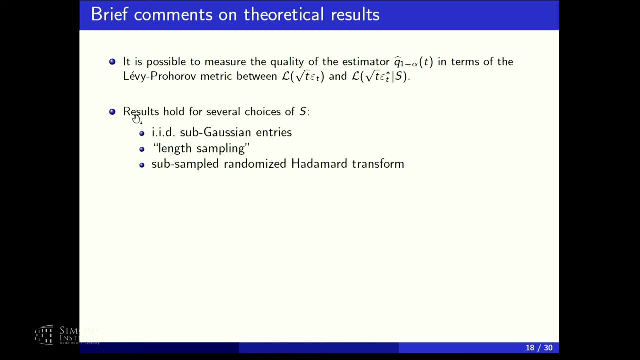 This is just sort of a technical thing And the types of sketching matrices for which the theory works. There's a variety. You can do iid sub-Gaussian. It's maybe somewhat idealized but still interesting. You can do length sampling. 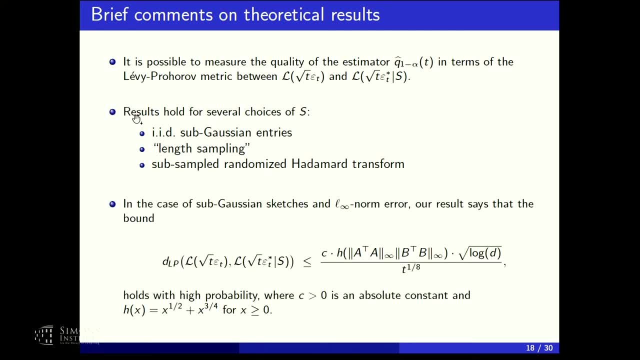 And the theory also applies to randomized Hadamard transform. Here's what one of the results looks like in the sub-Gaussian case. just because it's a little bit simpler, I'm using the entrywise maximum absolute value norm as my norm for the error variable. 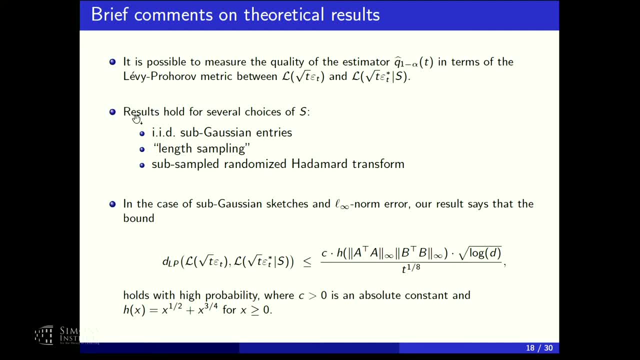 OK, Certainly we could talk about exploring other norms. But even As simple as that norm may seem, the theory is surprisingly involved, And this is what the distance between the bootstrap distribution and the actual distribution looks like with high probability. So this distribution here on the right, that's a random probability distribution. 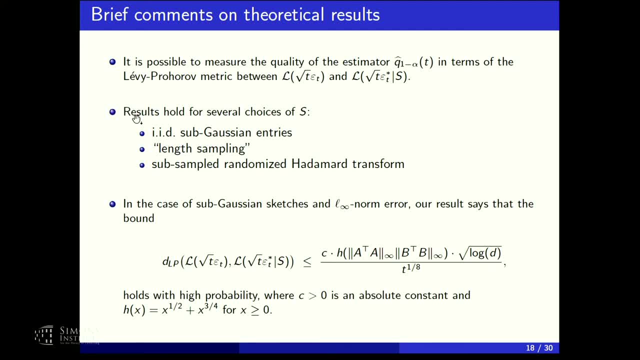 Therefore, this distance is a random variable And I can concede that maybe in the context of numerical linear algebra, the shape of this bound might look a little unusual. In the high dimensional statistics literature, when analyzing problems involving multiplier bootstrap methods, this type of bound is actually not so uncommon. 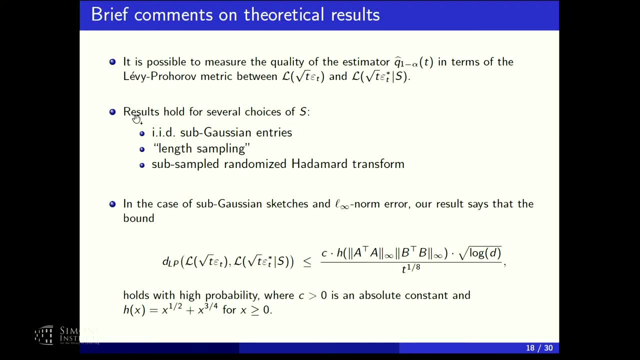 So I think it's important not to take the exponents in too literal of a sense, I think, at a first pass. the way to think about this is: there's a problem-dependent scale factor, There's a dimension-dependent factor And there's a sketch size. 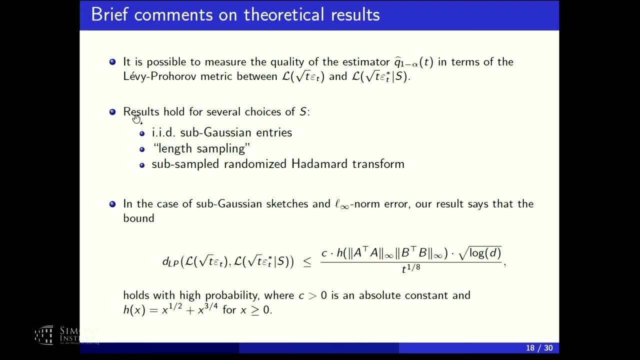 And basically The result at a minimum is telling you, as long as the sketch size is sufficiently large compared to these other two factors, the bootstrap's going to work OK. So Excuse me So if I go ahead at the beginning of my experiment and divide all the matrix entries by a million, 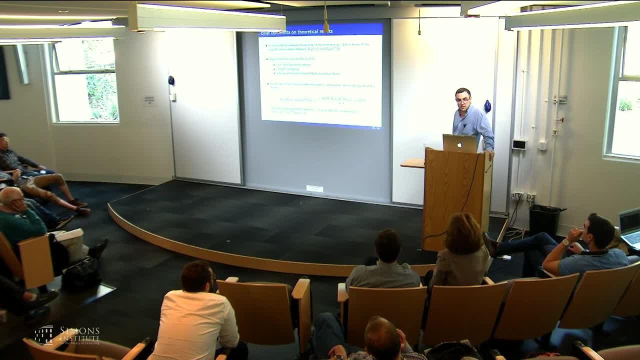 Yes, Right, Then that bound looks a lot better, doesn't it, Indeed? So I mean it's natural that you should have a problem-dependent scale factor, Because I mean, if you change units, it's going to be, you know, if you use, if you. 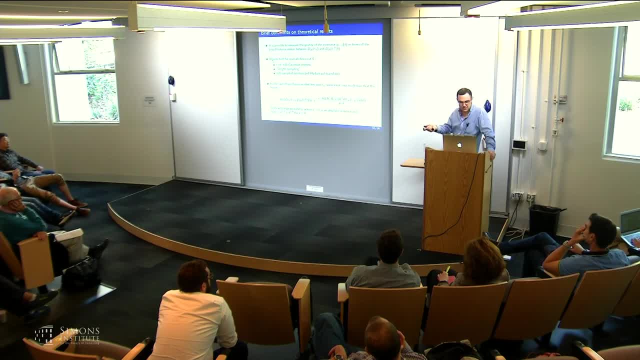 blow everything up, it's going to be a lot harder to get a good accuracy. So yeah, I mean, I think maybe it would be similar if you scaled things so that these norms are one even I don't think this is something to worry about too much. 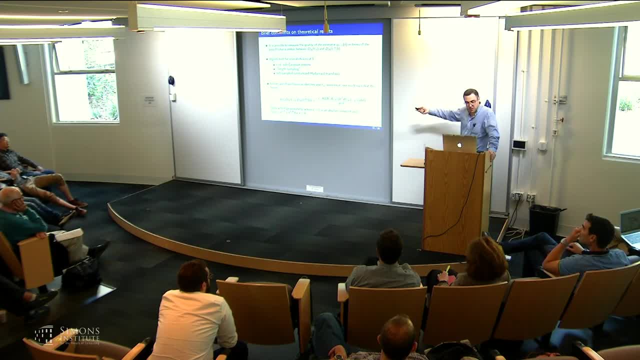 But I think it's not unexpected that there is a problem-dependent scaling factor. Do you think one can fix it? Yes, And also, I mean this function h is a little bit. you know Where does that come from? Why is that there? 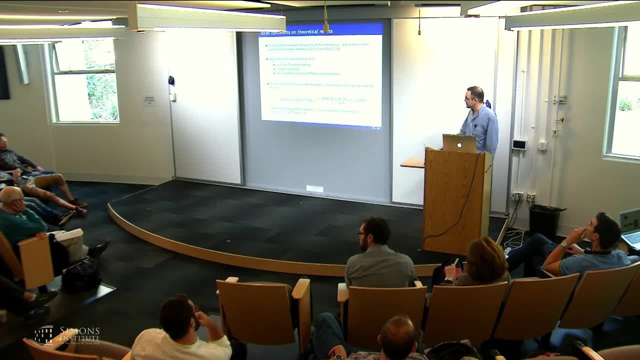 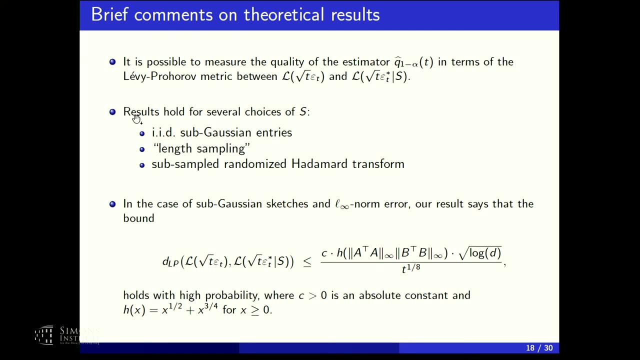 So let's not spend too much time on this. There's a lot of other theory in the paper that I'm not going to talk about, And also, I mean there's some interesting ideas that I wish I could talk about, which I think are novel contributions. 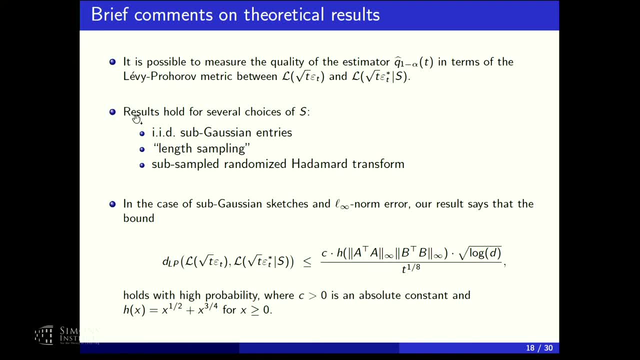 But in the interest of time I'll skip over all of that. What is that distance? Oh right, So the Levy-Prahorov metric, So there's actually a variety of, there's a whole bunch of probability metrics, Or metrics on probability distributions that you can think about. 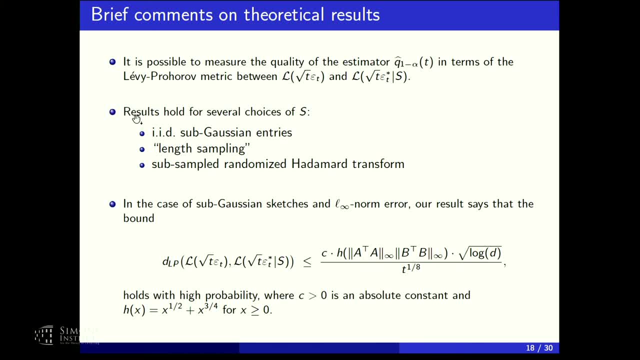 They all have different advantages and disadvantages. This one is a particularly nice one because it metrizes weak convergence. So a sequence of random variables converges in distribution if, and only if, the distributions converge with respect to that metric. So this is sort of a natural one. 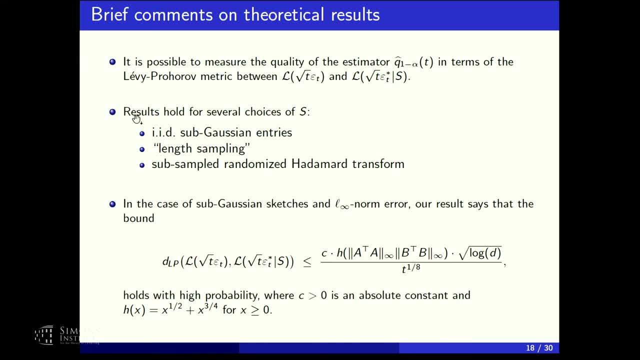 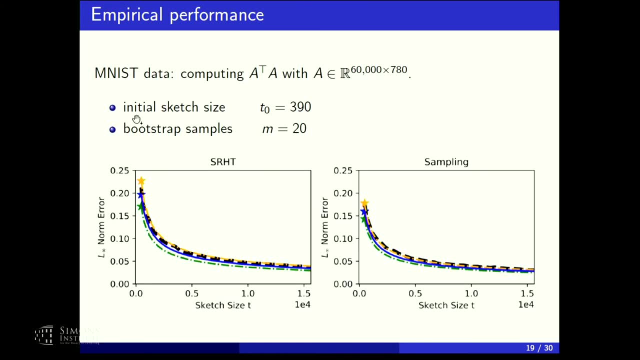 And it also relates naturally to quantiles. But that's a minor point, OK. So let me say something empirical, OK. So I think in some ways this is one of the more exciting slides. So here's what's going on. 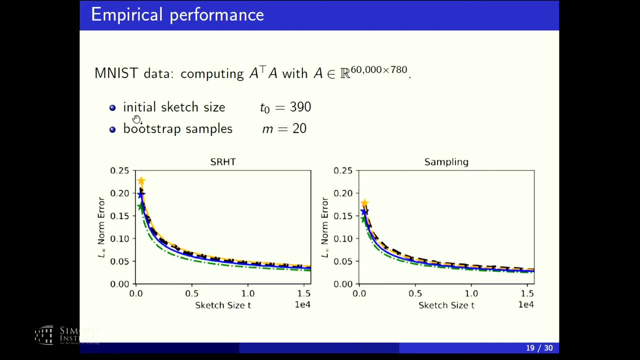 The two plots just refer to two different kinds of sketching matrices. So the experiment on the left involves randomized Hadamard transform. The experiment on the right involves length sampling. My full matrix A has 60,000 rows and about 800 columns. 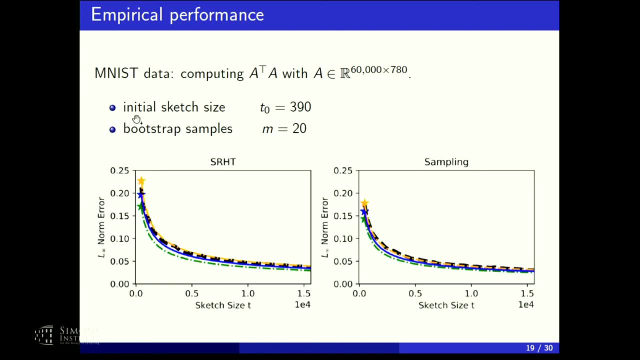 I'm using an initial sketch size of 390.. That was chosen just because it's half of D, So 390 is obviously a lot smaller than the full number of rows- 60,000.. So that shows you that you can really start out with quite crude sketches. 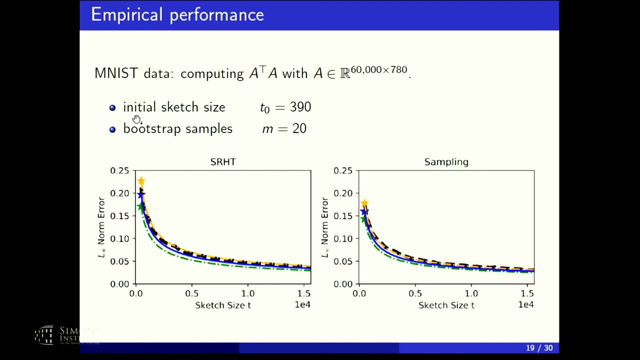 The number of bootstrap samples, as I mentioned earlier, I'm going to take to be 20.. So really, what's going on is I take two really small sketches, I apply the bootstrap. The black curve represents the true quantile function at every t. The blue curve is the 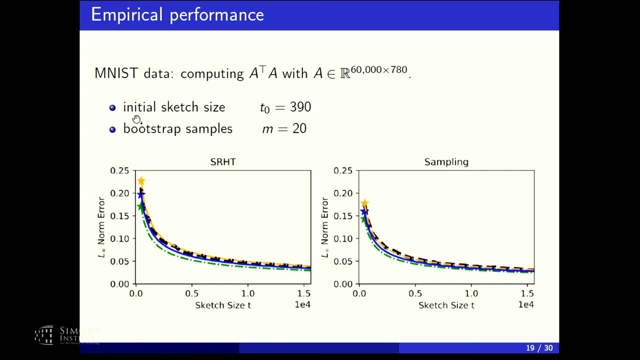 mean of the bootstrap s. The blue curve represents the true quantile function at every t. The green and the yellow are one standard deviation away. So here is where the bootstrap actually gives us one estimate, And the rest is all from the extrapolation rule. 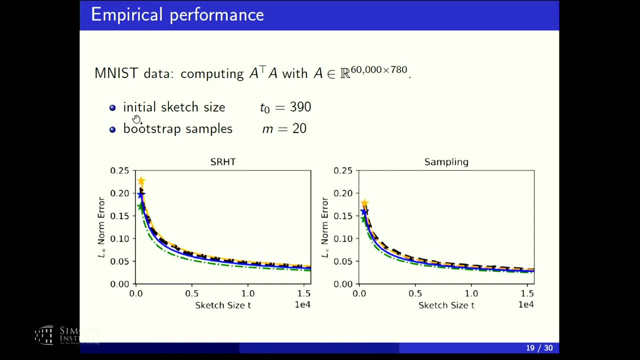 So I think this is kind of remarkable, that we can predict quite accurately what's going to happen well past 10,000, starting out with only 400.. So the extrapolation is a really useful thing And again it works kind of regardless of what kind of sketching matrix you use. 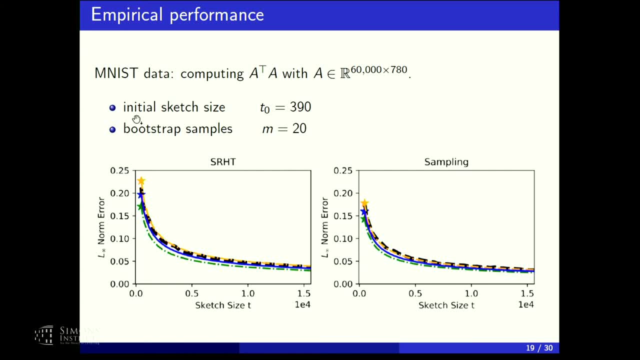 I mean there is a little bit of dependence. You can look at those details in the paper, But more or less the details of the sketching matrix are not so critical. So if you took that experiment and you rescaled, like Lisa suggested, by 1 over 1,000.. 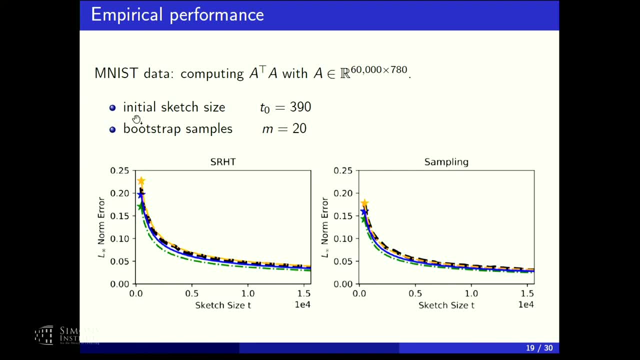 Yes, So, indeed. So I forgot to mention in this experiment we scaled the Gram matrix, so the largest absolute value is 1.. Oh, OK, So indeed, Yes, Yes. So just to put this in context: if I just estimated 0,, how much error am I going to? 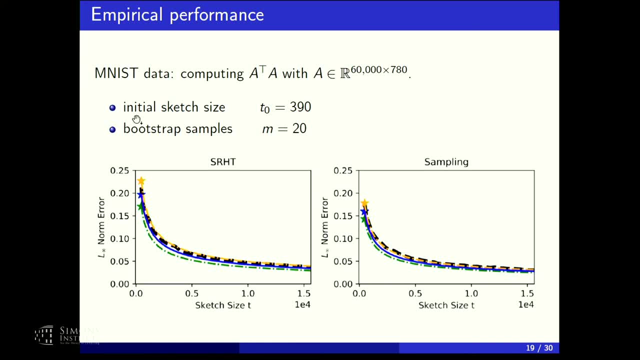 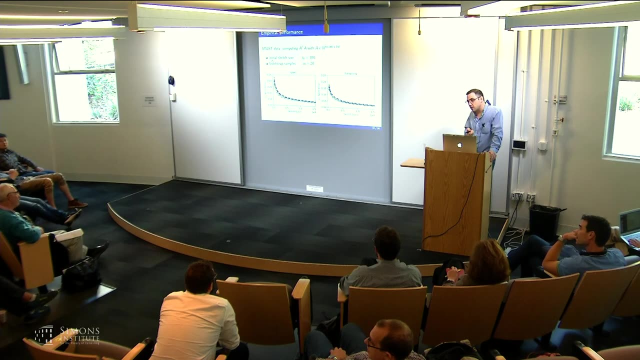 get 0. 0. Like is the error going down just because the expected error is going down as well. So you're saying if the A matrix is 0? No, no, If I estimate how much error I'm going to get between A tilde B. A tilde transpose B. 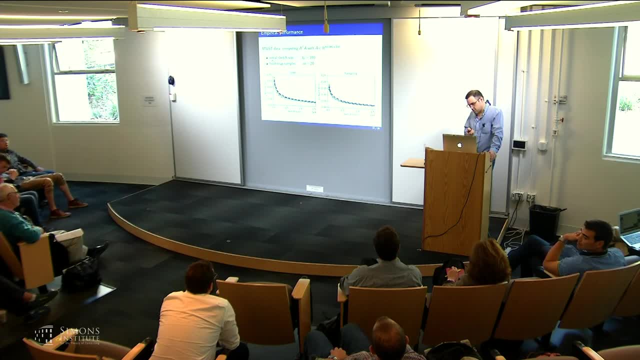 minus A, transpose B right, and I just estimate that error is 0, is my plot going to look like this Or is it going to be dramatically worse? Uh, Yeah, So I mean in fewer words. are you asking if the estimate is vacuous? 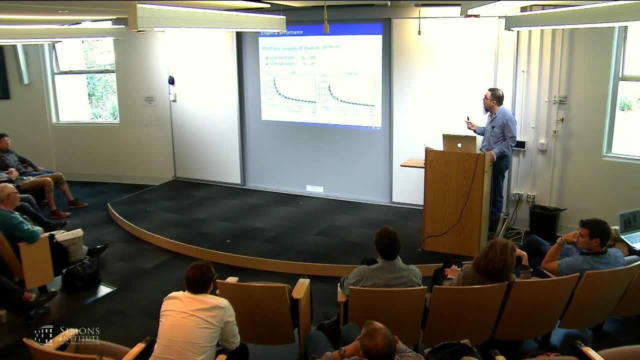 I don't think so. I mean so I need to think for a few minutes to give you an accurate answer to that, but I don't think 0 is going to work. Yes, So assume A and B have some structure- assumption OK, which we're often hiding. 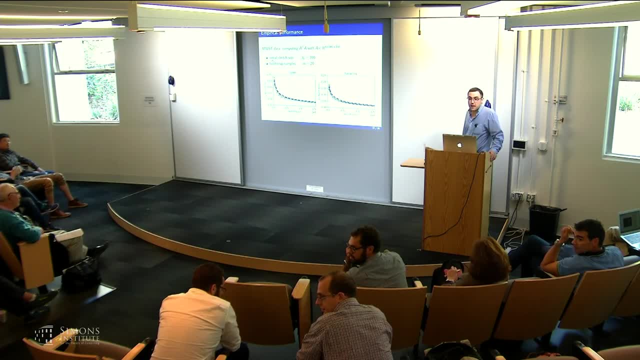 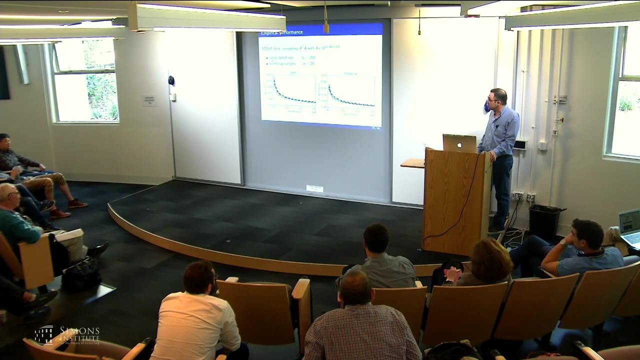 OK. Is there any way to design some sampling scheme or projection random sketching matrix to respect that structure? Is there any way of doing that? There's a lot of things that could be done with it. That's a good idea. What's nice about the bootstrap is that in a lot of ways it's agnostic to the structure. 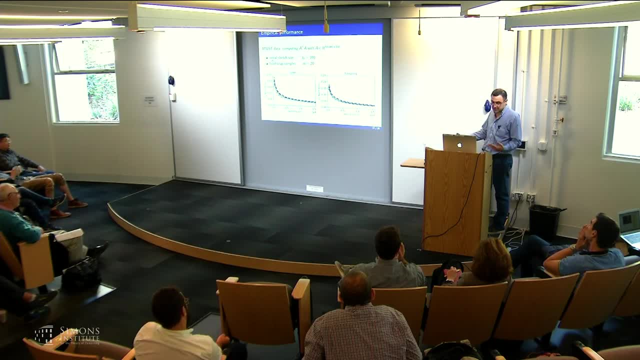 of the matrix. It works reasonably well for a lot of things. I imagine there's possible improvement that you could get in structured cases, but that's something I haven't looked into in detail. OK, So I don't actually have a lot of time left. and there's still the entire least squares. 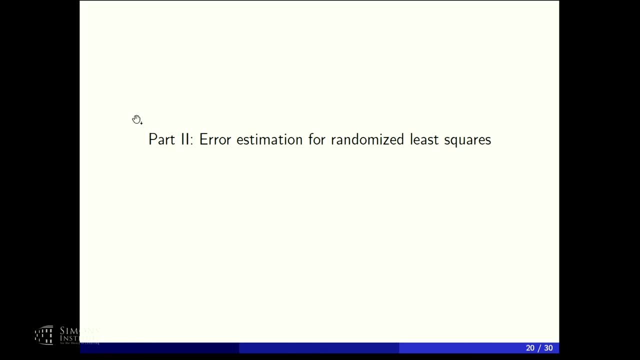 portion. So just bear with me and I'll try and get through the important points quickly. OK, So in the least squares case I'm going to look at a tall A matrix, a long B vector, and I want to solve an overdetermined least squares problem. 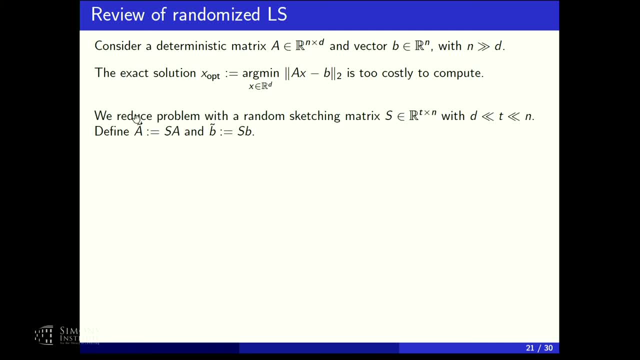 Again, n is much, much larger than d. I'm going to use the sketches And an important point is that, OK, there's more than one, There's more than one type of sketching algorithm you can use to solve this problem. 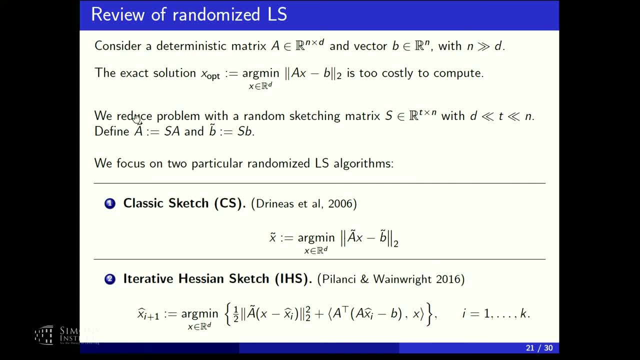 There's the sketch and solve kind of thing. due to Jornet, Mahoney and Muthukrishnan, There's more recent proposals that are sort of more like quasi-Newton methods. But what I think is really interesting is, even though these algorithms are quite different, 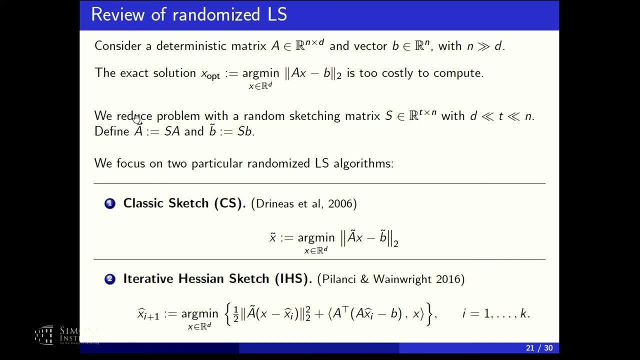 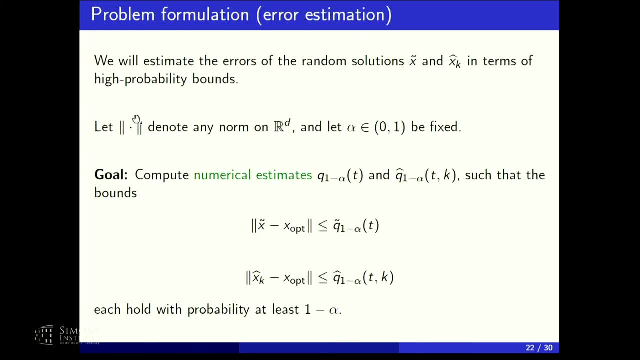 the bootstrap still accurately estimates the errors of either of them. So you get to take your pick and the bootstrap will still do its job, OK. So I think that's enough here, OK, So the formulation I'll think about in the least squares case is pretty much the same. 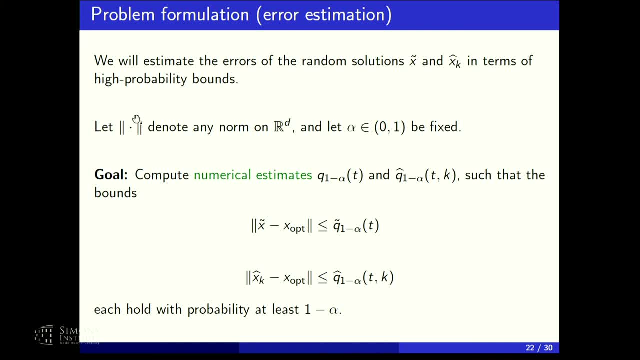 I want to estimate the quantiles of the error variable. OK, Now again you can pick some norm on the solutions. The quantile function will depend at a technical level on that norm. But let's not worry about that for now. 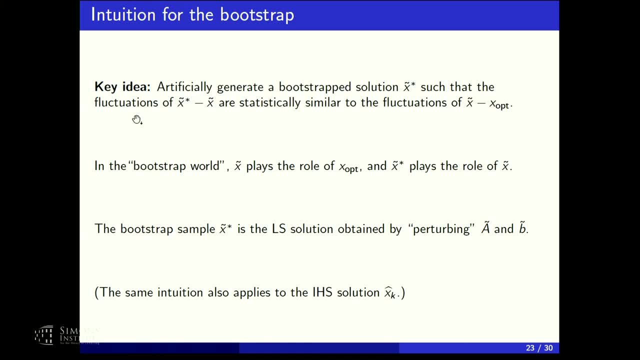 OK. So we have this intuition for the bootstrap that we're generating pseudosamples In the least squares case. I think a nice idea to keep in mind is that you can think of the bootstrap as doing something sort of in a parallel universe where the original 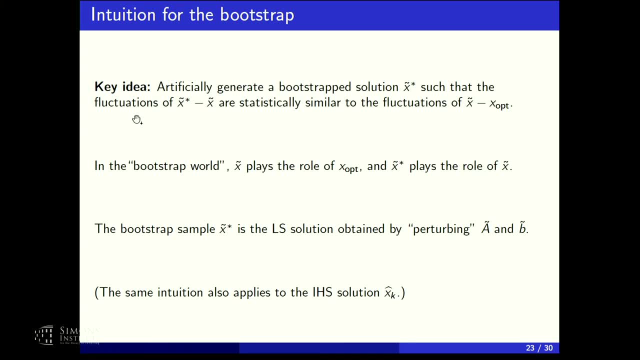 sketch solution in the parallel universe is playing the role of the true, exact solution And the bootstrap is sort of constructing this perturbed kind of scuffed-up version of the sketch. And if the difference between the scuffed-up version of the sketch and the sketch is statistically 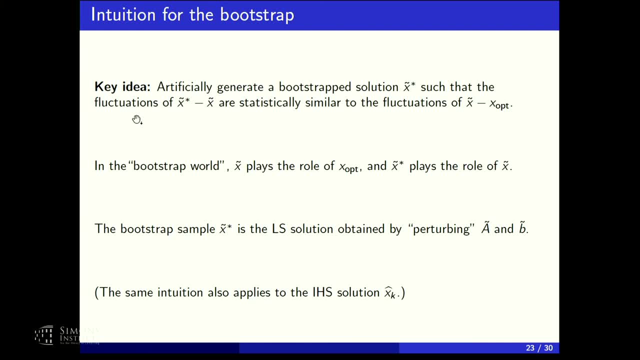 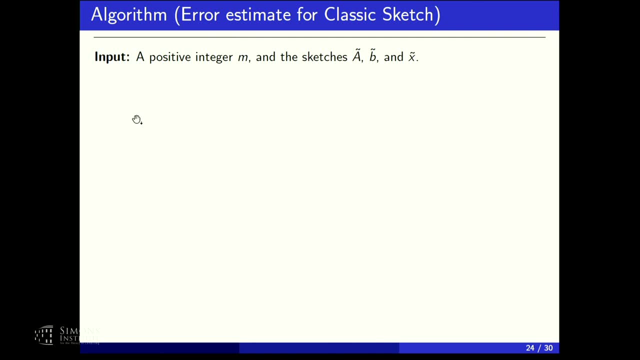 similar to the fluctuations of the actual error variable, then that's a way of thinking about the bootstrap, and if it is doing its job, OK, Here's the algorithm. So this is more or less the same template that I described for the first version of. 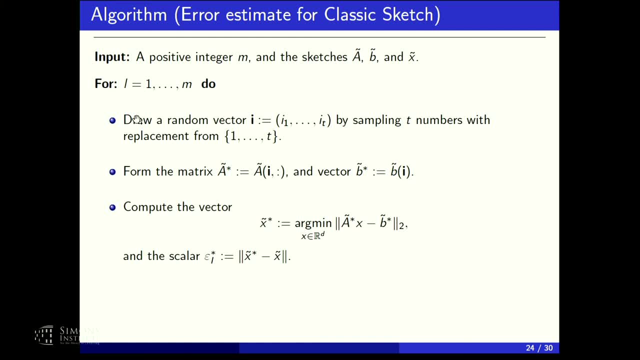 the bootstrap. So I'll draw t numbers with replacement from the index set 1 through t. I'll use those indices to extract a new set of rows from the original sketches or entries of the vector b tilde. I'll solve the associated least squares problem with the starred inputs. 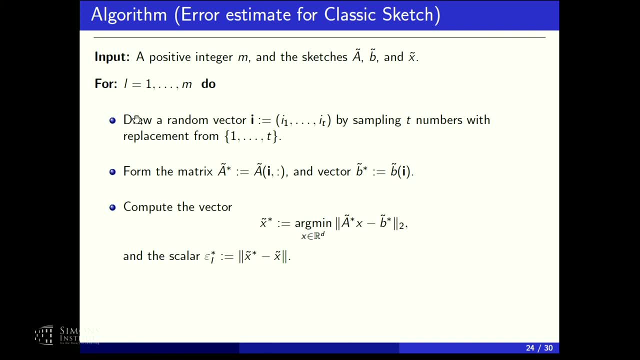 OK, That will give me a starred solution. OK, And for that particular iteration of the loop, that will give me one bootstrap sample by taking the norm of the difference between the starred solution and the unstarred one. Then, after I've done m iterations of the loop, I'll again take the desired quantile of those. 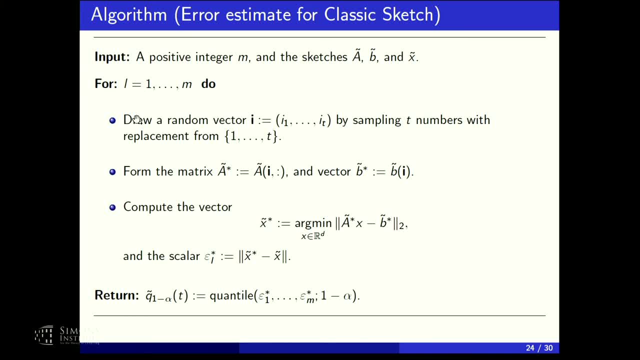 numbers. OK Now, the Gaussian multiplier bootstrap that I described earlier actually is not appropriate in this setting. It is important that I do the sampling without replacement in this setting, but that's just something to mention. And one other thing is that this template more or less works in the same way for the 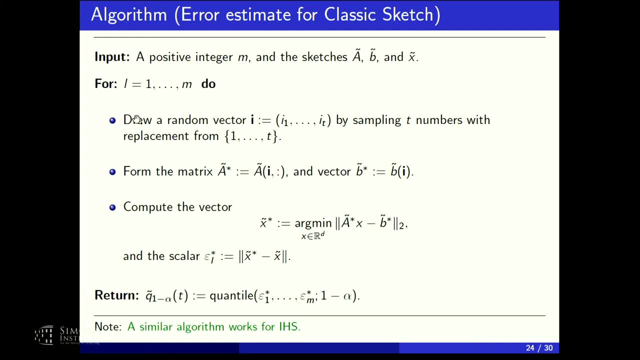 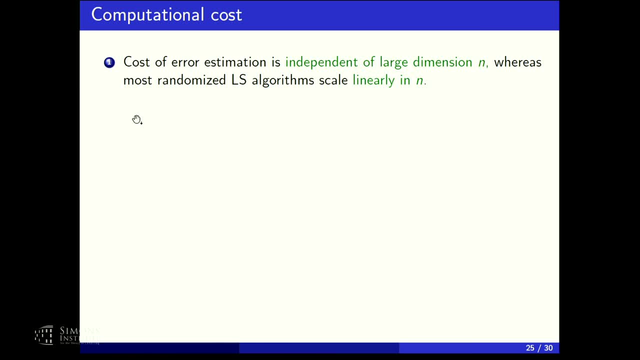 iterative Hessian sketch algorithm. There's a few minor details that have to be modified, but it looks more or less the same Computational cost. A lot of the same high-level remarks apply again. So one important thing is that the cost of the bootstrap is independent of the large 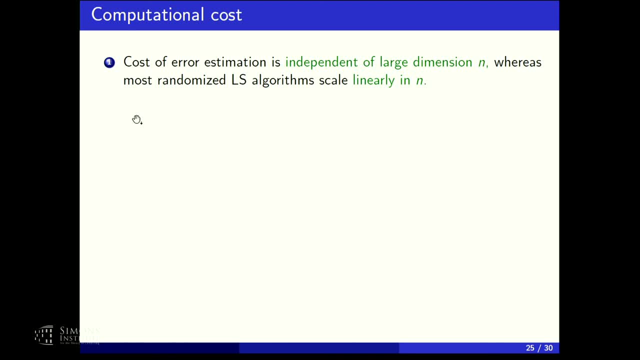 dimension n. That's great because it means it's highly scalable. But it's also very important that the cost of the bootstrap is independent of the large dimension n. OK, And there's an easy way to see that: just because the bootstrap never sees the full 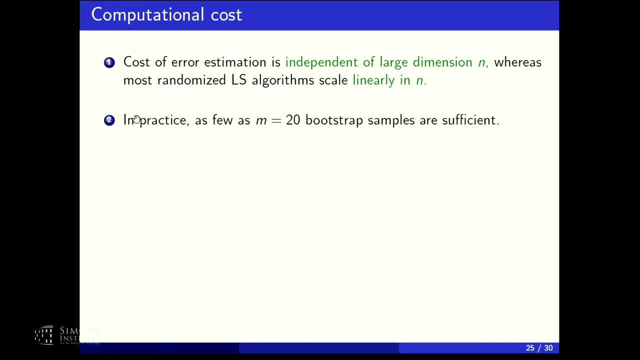 inputs. It only sees the sketches Again. in the least squares case, 20 bootstrap samples is typically adequate. I didn't mention this detail before, but the bootstrap samples can be generated in an embarrassingly parallel manner. None of the bootstrap samples have to talk to each other. 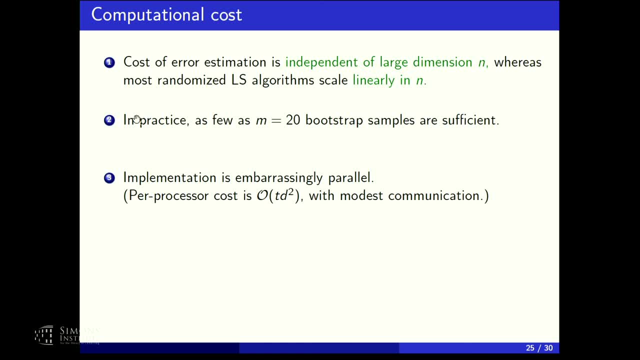 Furthermore, the communication cost is pretty small because you're only communicating the sketches, And in fact it's even better than that because you're only communicating the initial sketches. So those are quite small matrices. This is something you could do on a laptop perhaps. 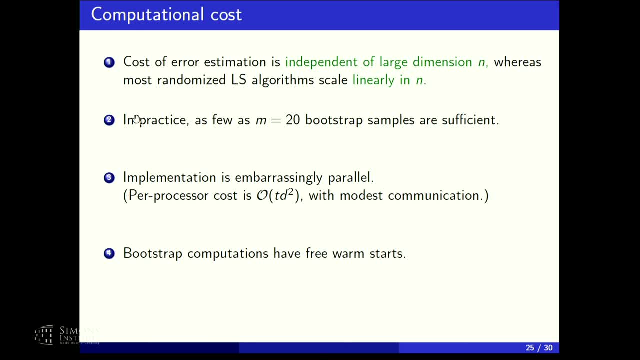 And even better, in the least squares context, the bootstrap computations have free warm starts, because at each iteration of the bootstrap loop you're solving a new least squares problem. The bootstrap solution is going to be close to the original sketch solution And therefore you can use the original solution as a warm start if you choose to. 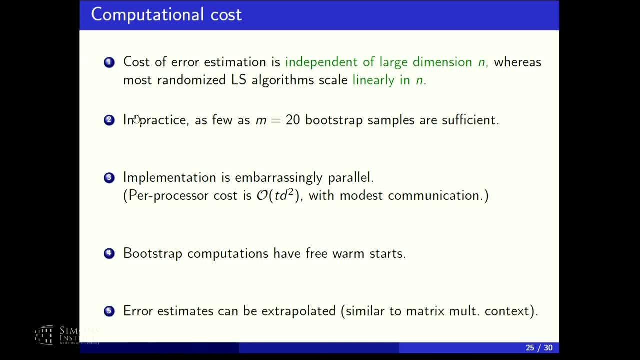 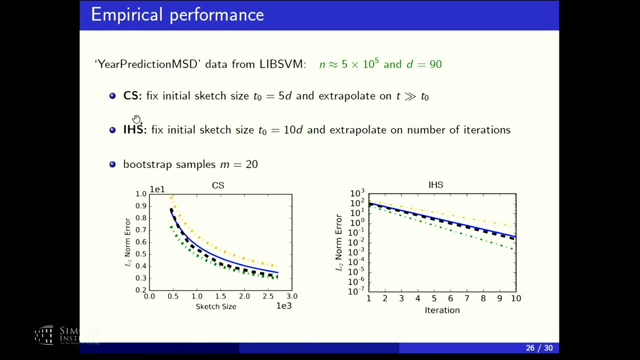 Can you wrap it up? So right, So. So here are some plots. I'm using extrapolation here. as before in the iterative Hessian sketch, I'm going to use a linear extrapolation rule rather than the square root of t rule. that.